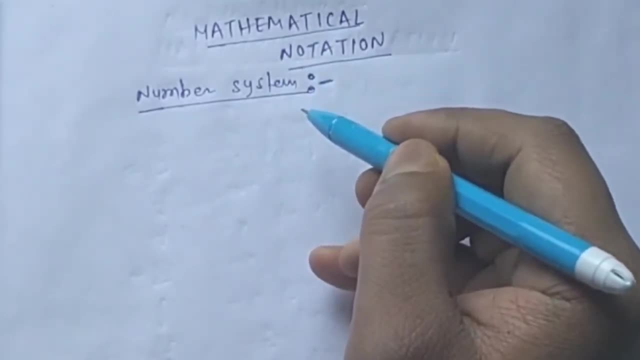 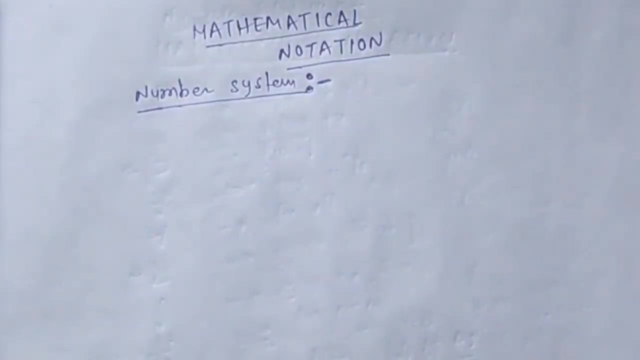 After that we will discuss further, Because all these things are basic things. If they can't understand, then there is a problem In completing the mathematical part, Because when you read any book, So there these types of symbols are repeated again and again. 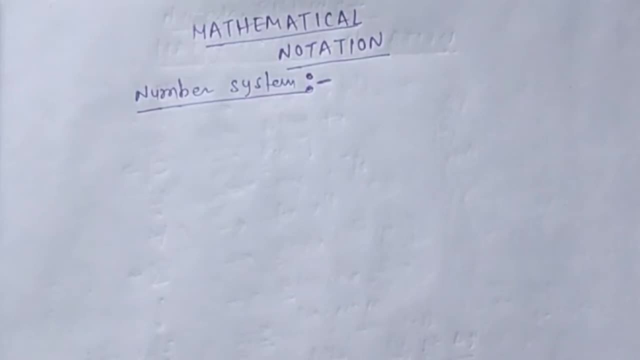 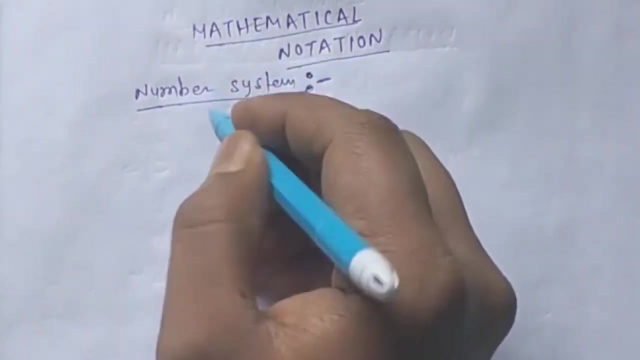 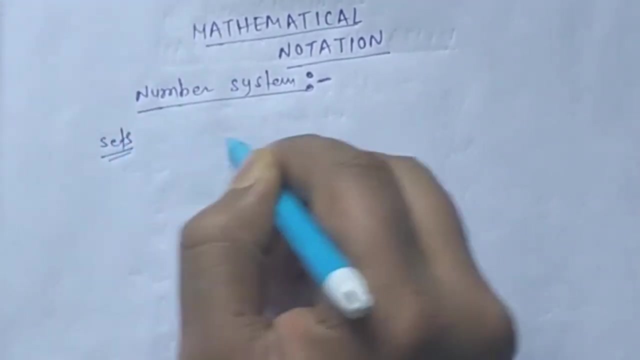 So we have to understand those terms So that we can understand that line completely, What he wants to tell in it. So first of all we see that we read sets, So we had a lot of types of notation in sets. You must have done this in 9th and 10th. 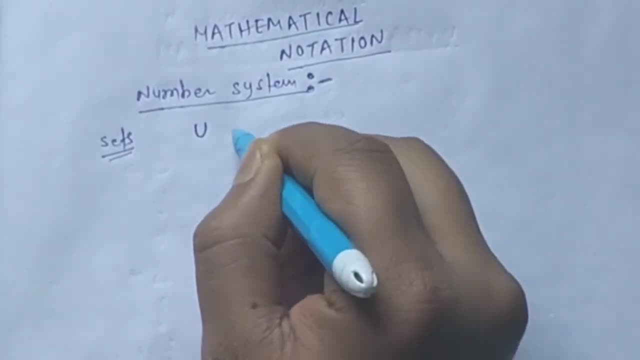 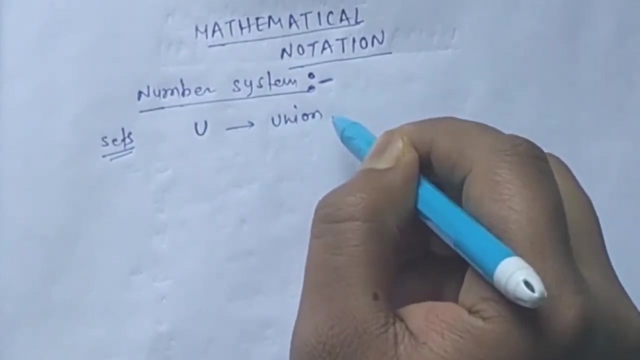 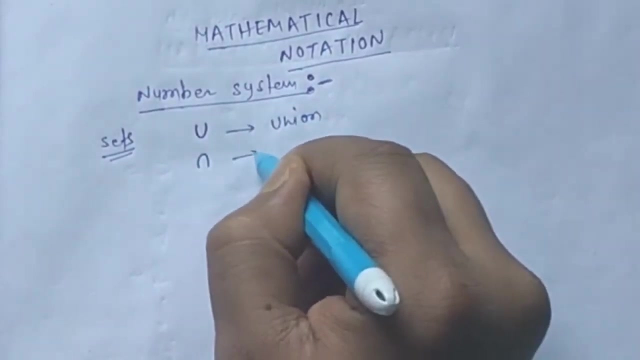 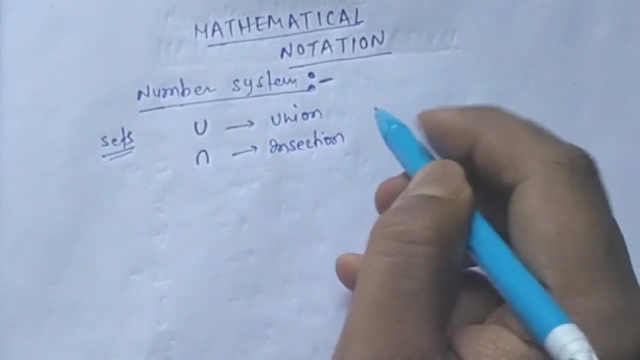 We have this type of symbol. What do we call this Union? Similarly, what does union mean When we combine two sets together And what is this Intersection? So this is our intersection. Apart from this, And we have one notation- 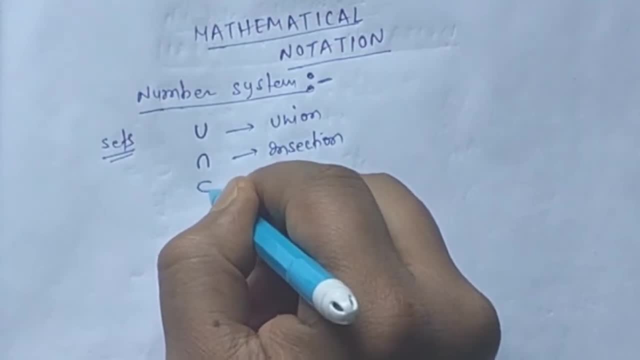 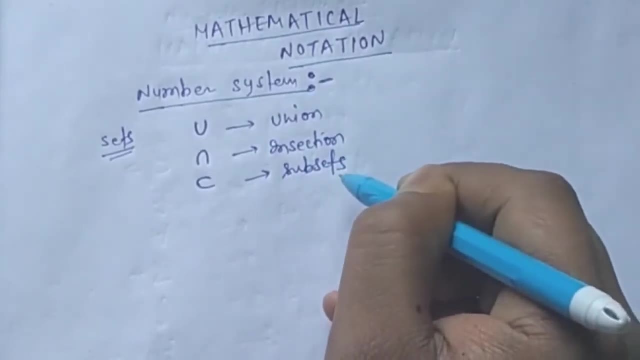 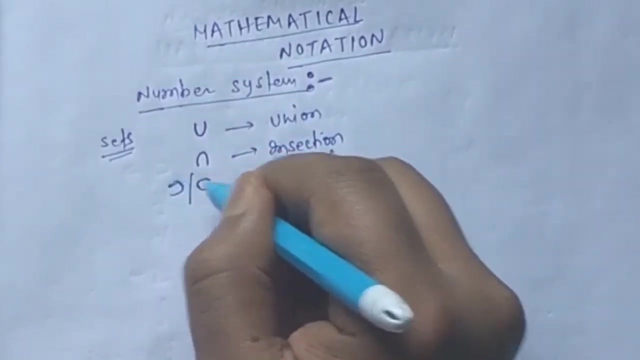 This type of subset, Isn't it? We used the symbol of subset. You can call subsets, Isn't it Subsets or supersets? Both these types of symbols are used. Any symbol, It depends on what our question is. Apart from this, we have 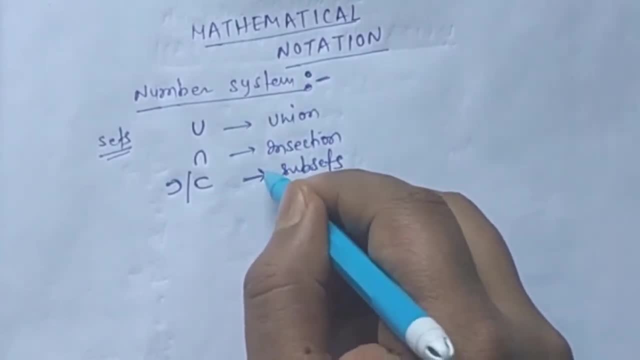 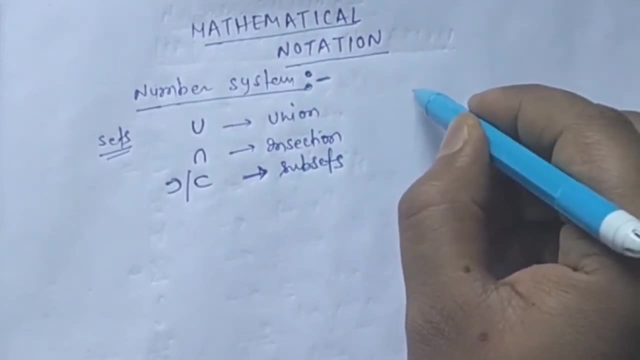 There were more symbols, As we can also subtract in sets, So in that subtraction is the same symbol. Here you will pay attention to one thing, That same thing when we, When we studied this in Algebra And in Mathematics, When you study normal Mathematics. 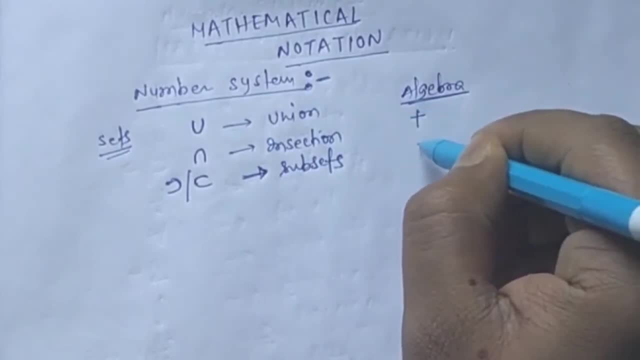 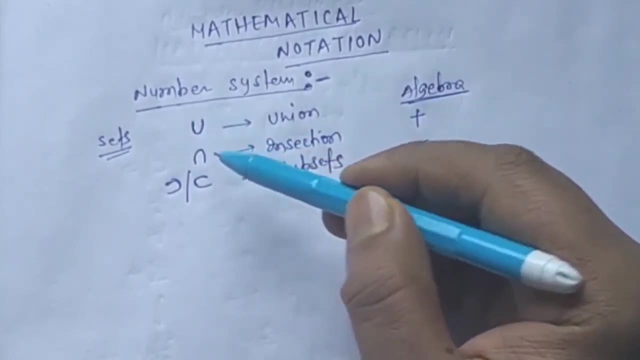 There we have For sum, For plus sign, For subtraction, For minus sign, Isn't it? We used this? But here also, What is union? In a way, it is addition only. So for both of these, Why did we use different symbols? 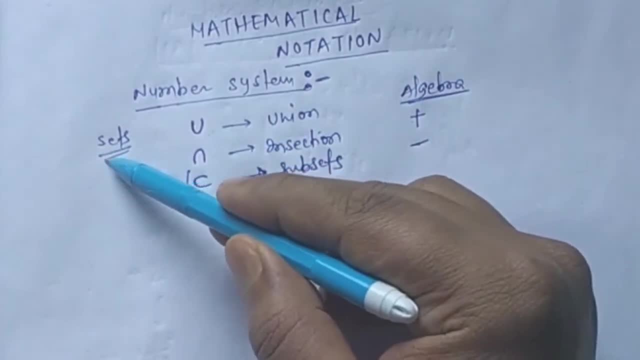 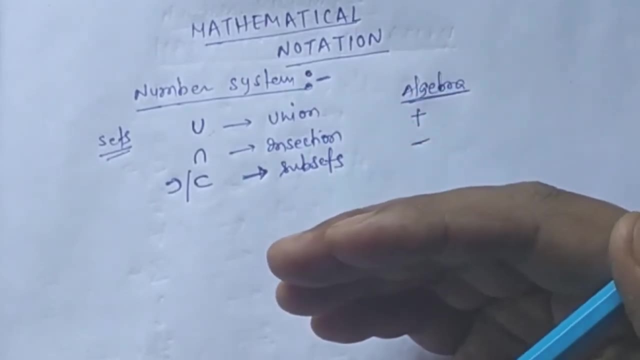 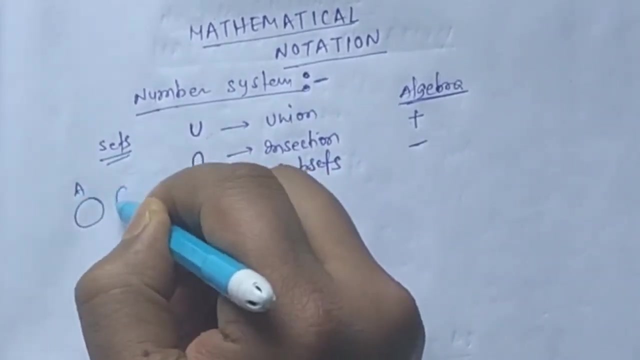 So the union happening here, The union in sets. What I am doing is That these Two Types of We can say this: Like we have some, This is a set And this is a set, Isn't it? So what is set in itself? 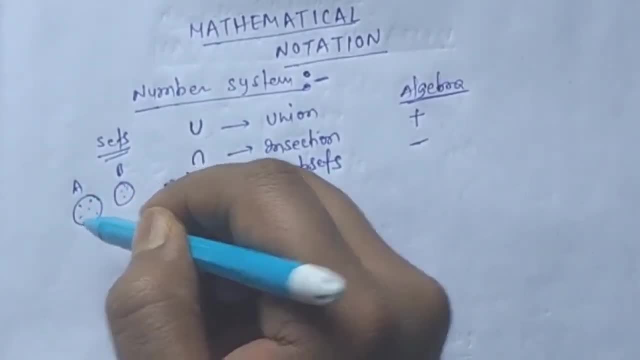 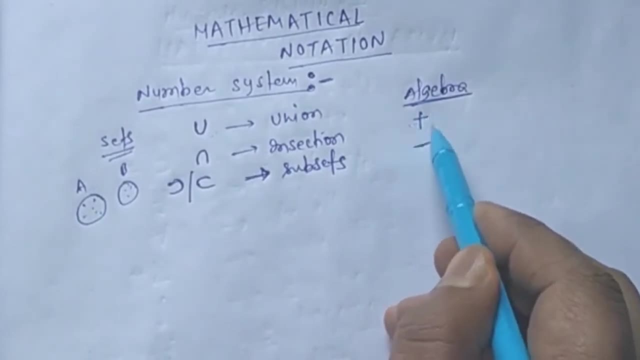 Collection of objects. Here we don't deal with one object, We are dealing with many objects together, Isn't it So because of that, We don't use the same symbol. Where is this symbol used When we have to add single, single elements? 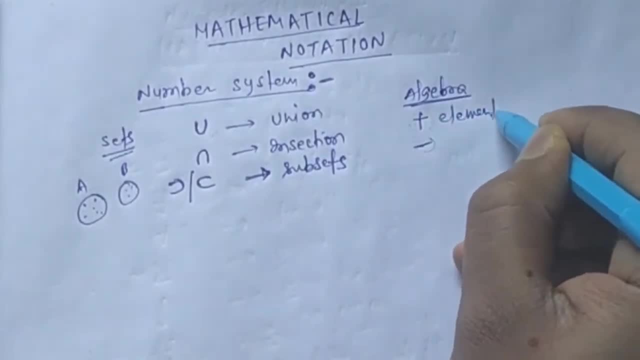 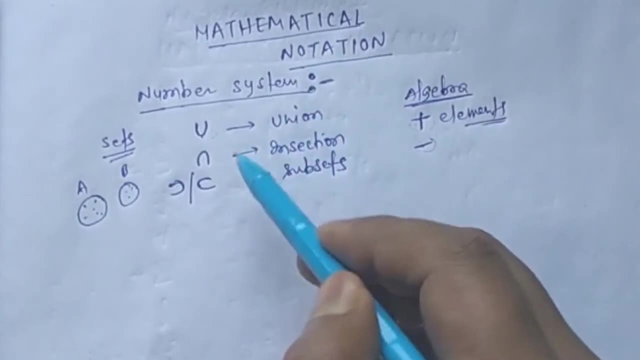 Isn't it So, this Of elements, The symbol to add elements, And this symbol, The symbol to add the collection of elements? Isn't it Similarly So? all these things? You already know. We just highlighted it After that. 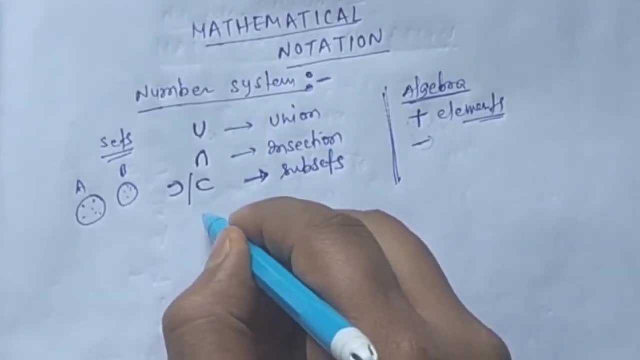 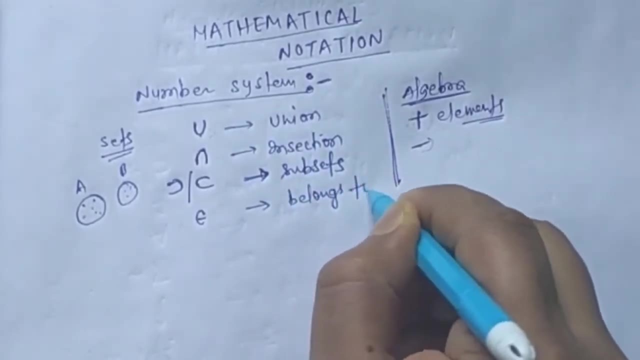 We have. Which other symbols are there? One: We saw this type of symbol, Isn't it In sets? What do we call this? Belongs to When one element, When one element Belongs to a set. So we used this symbol here. 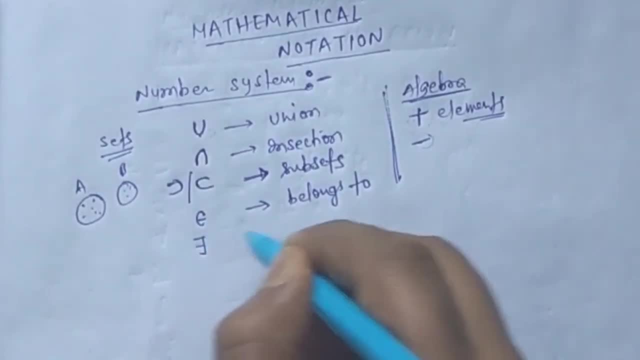 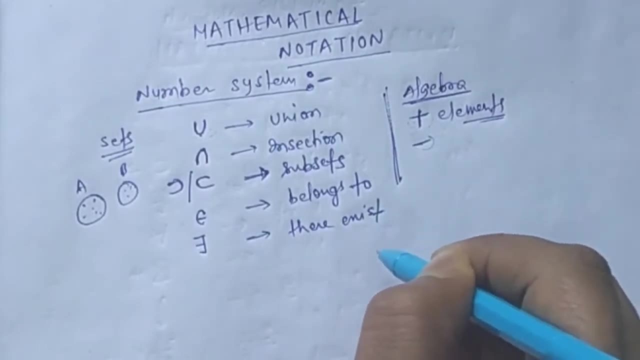 Isn't it? Similarly, Another mathematical symbol is used, This one. What is it called? There Exists, Isn't it? Similarly, One symbol. This is used. What is it called For? All Isn't it? So this is a mathematical term. 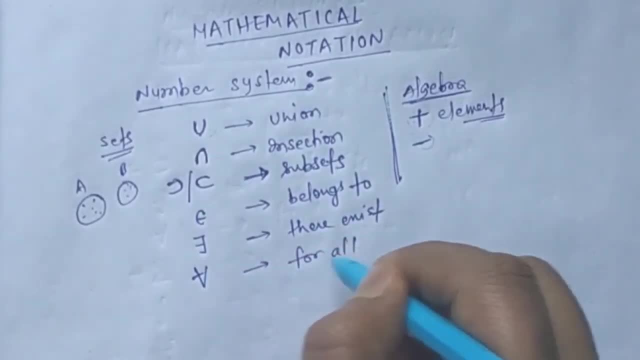 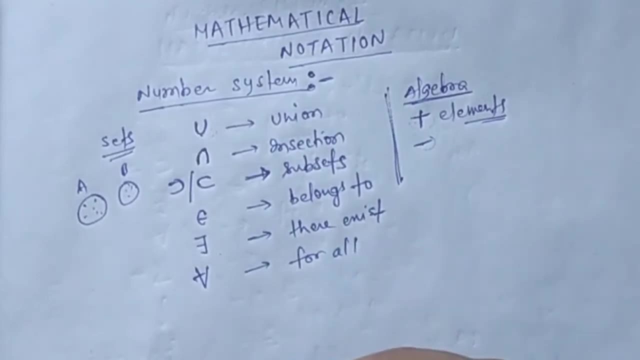 You will see somewhere That he, By not writing this For all word, Uses this symbol. So what does it mean? What we have to read? We have to understand This. We have to understand Similarly In sets, In the number system. 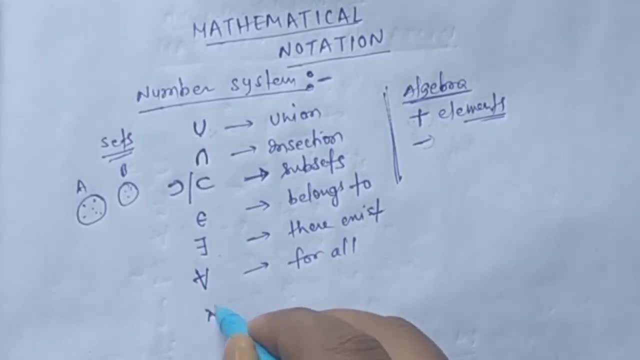 When we saw. So we used a lot of notation. N used, Isn't it? What does N denote Natural number. Similarly, We Decided Whole number Which we Donated from. W Denoted After that. 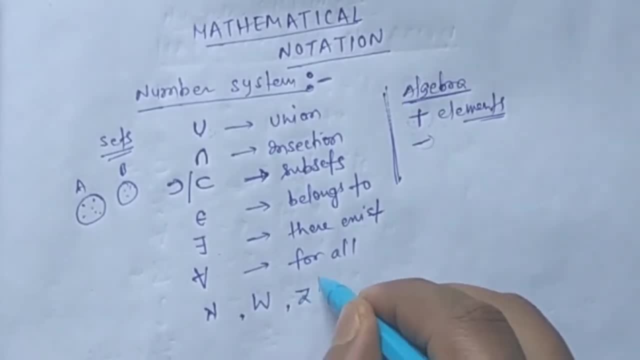 We have Integer Z And Which we Denote in the term of I. Apart from that, We have Rational number. Z Was Irrational number. Apart from that, We had Real number And Bigger than this. 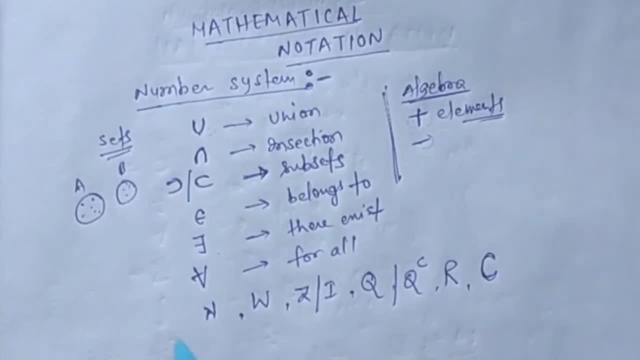 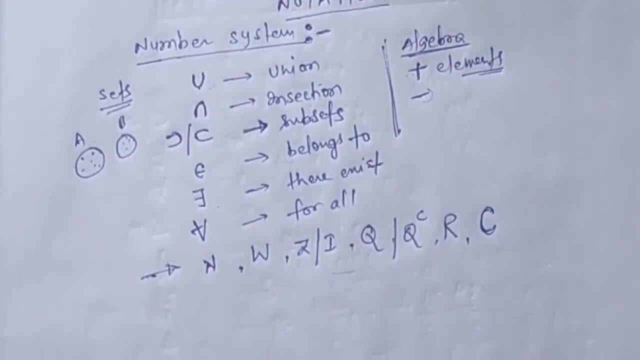 A set Of complex number. So we In the number System Part, We saw all this. That How We Different, Different Notations Denote one set, Isn't it? Apart from this, We have 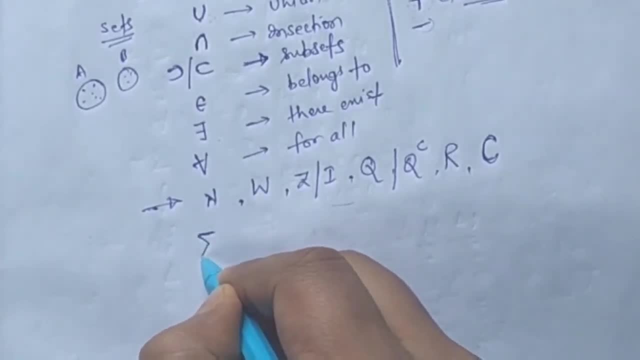 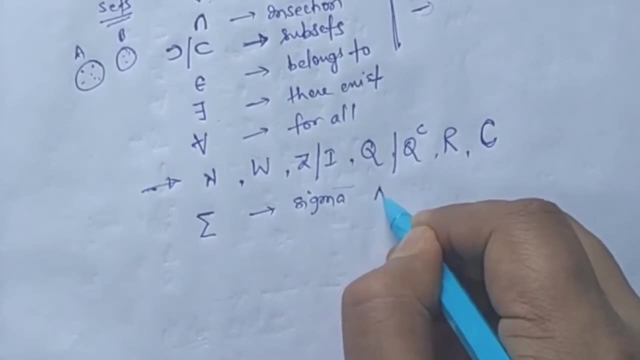 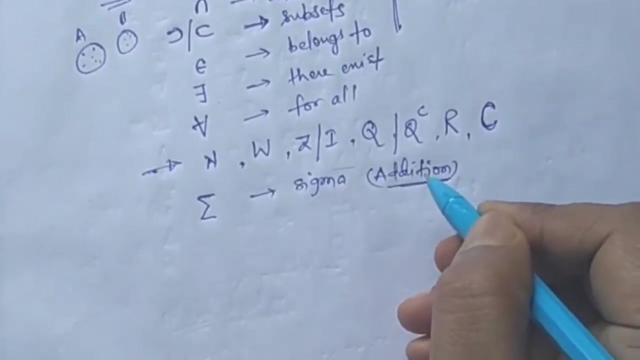 Some More Symbols Which you Have Of Sigma, What we Say Sigma And Its Work, This Addition, Okay, So Addition. Whose Addition Of Numbers Any Different? 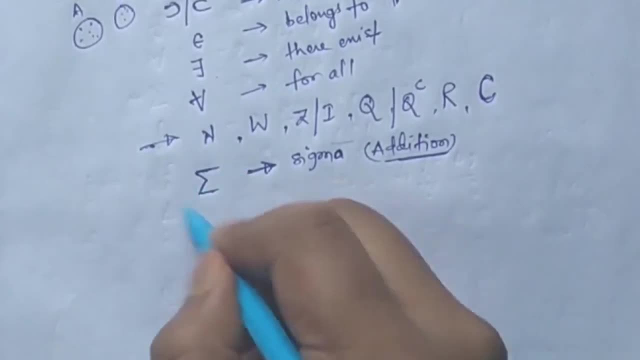 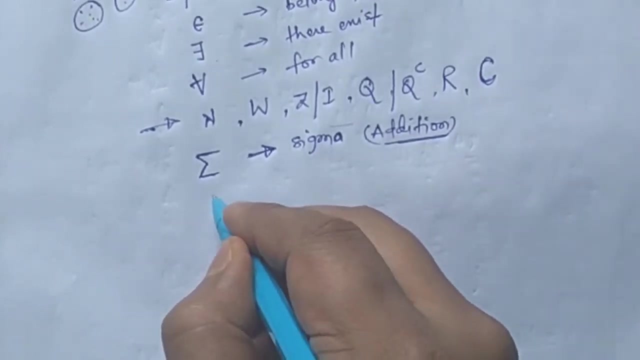 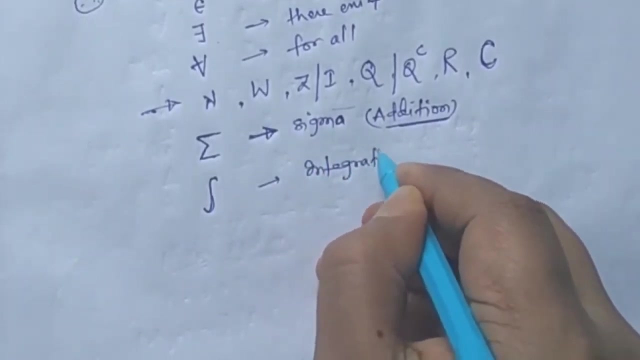 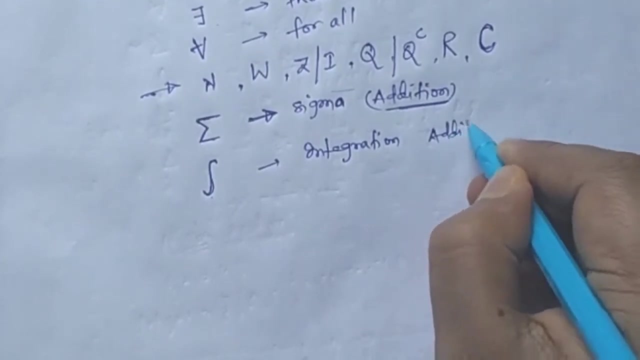 Different Types Of Numbers. We Single Single Types Of Numbers, As We Have One Symbol. This Is What We Say Integration, Isn't it About This, You? 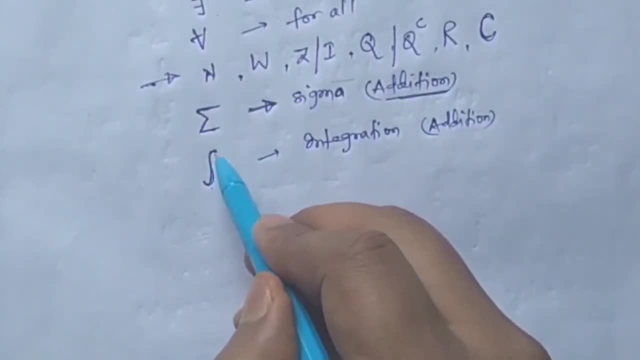 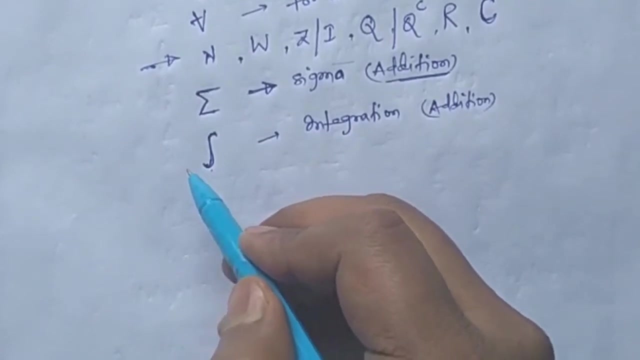 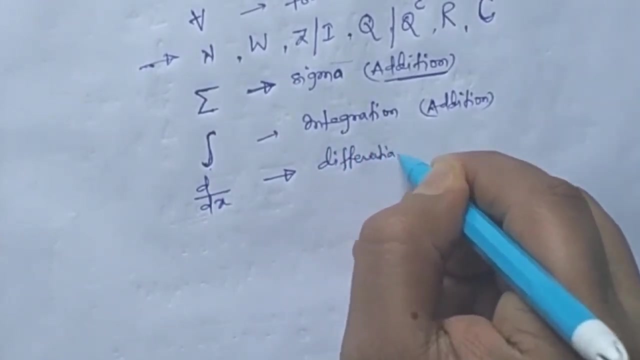 Will Read In Physics In Detail: What Does It Also Addition, Isn't it? But In Physics, In Mathematics, In Mathematical Tools, We Will Read This Part: 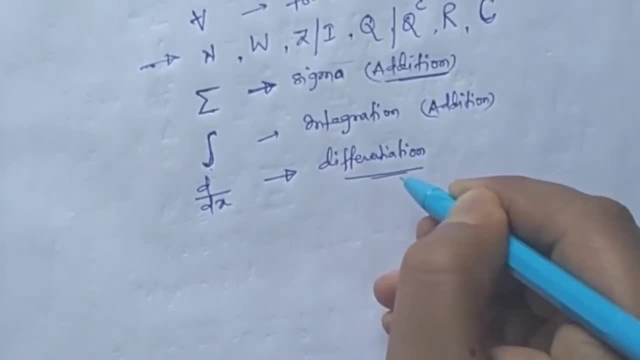 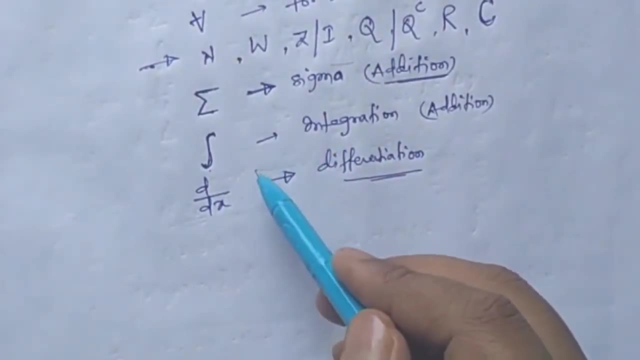 In Physics, In Mathematics, In Mathematical Tools Terms. We Will Read This All In Mathematical Tools In Class, In Neon Mathematical. We Are All Here To 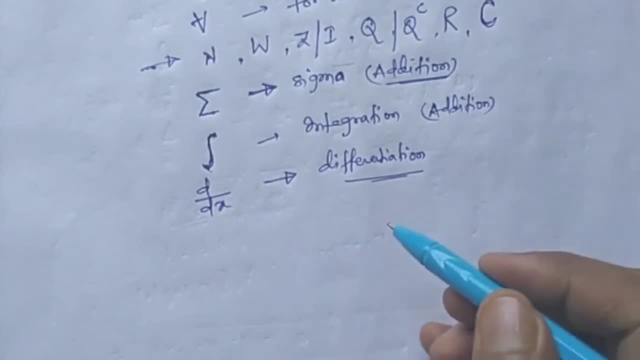 Read This, Chan. I want It To See Now. Screed The Sign Here's. I Will Diagnose That On Page 服 To He. what is the meaning of this? 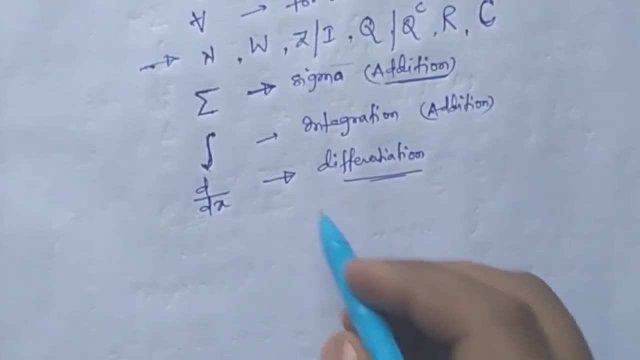 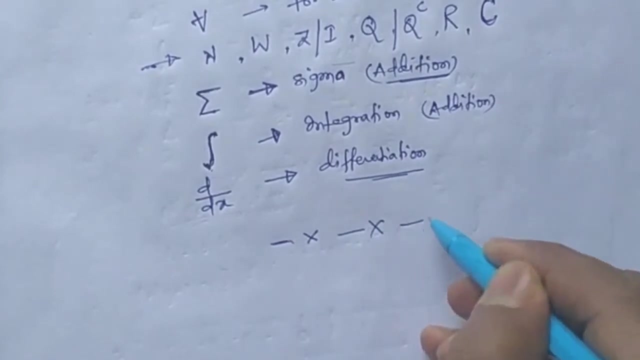 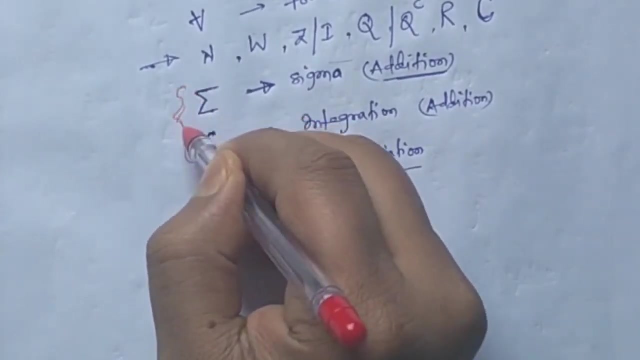 and if we forget somewhere, then we can revise this thing and check right. so this was so. apart from this, we will have many more symbols, so as the symbol comes, we will add it here. so now both these parts. once we check what is the meaning of these two. 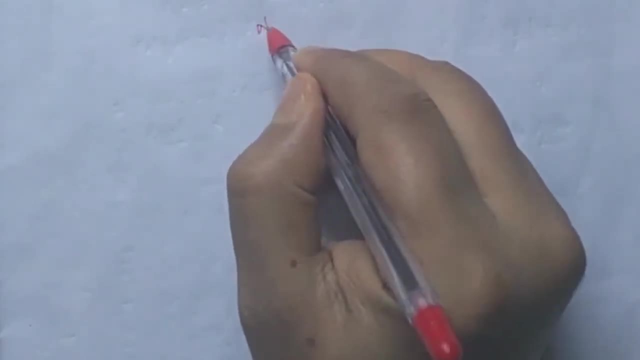 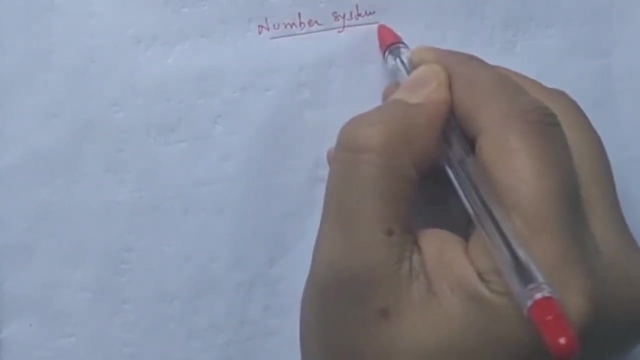 right? so once again, let's pay attention to the number system, right? so in the number system, whatever numbers we saw, we can divide all those numbers into two parts of a different type. we are creating a division. what we are saying to that division? suppose, if we have 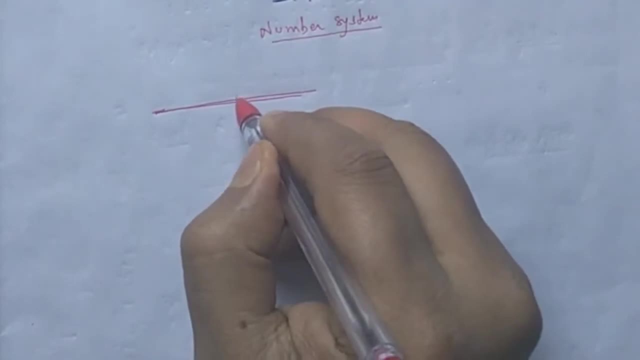 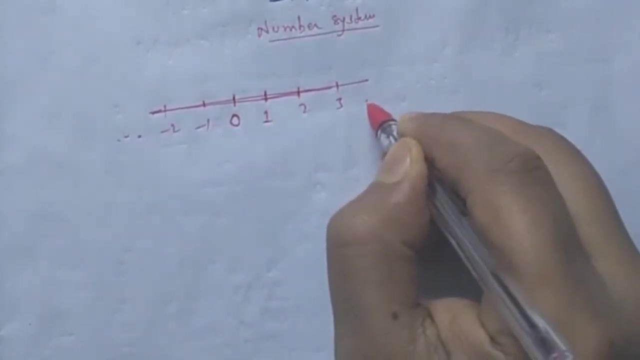 this number line and on this number line we have to denote 1. so where will 1 be? on the right side of 0, similarly 2 will be and similarly 3 will be, and on this side minus 1, minus 2, and from this type we move the number. 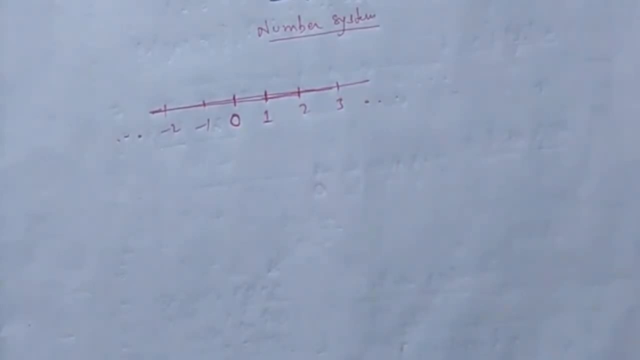 right- so you must be understanding all this- that we can denote any number on the number line. now, if someone asks us tell me where is 1, it will be only here. if someone asks where is 2, where is 3, from this type, we can do all the numbers. 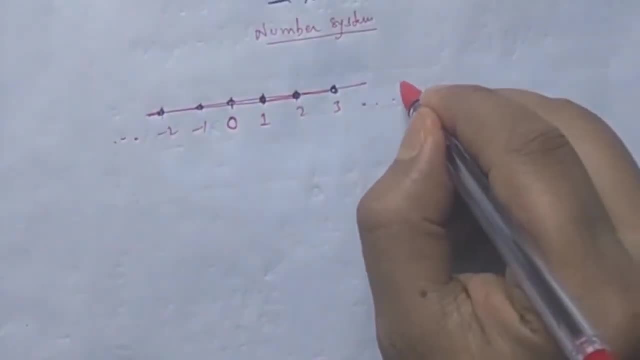 we can mark. now we are taking one more number line and in this we can count that this is the real line. so what happens in this real line? that every point of this line is denoting any number. so now, if someone asks you, tell me how many numbers are there. 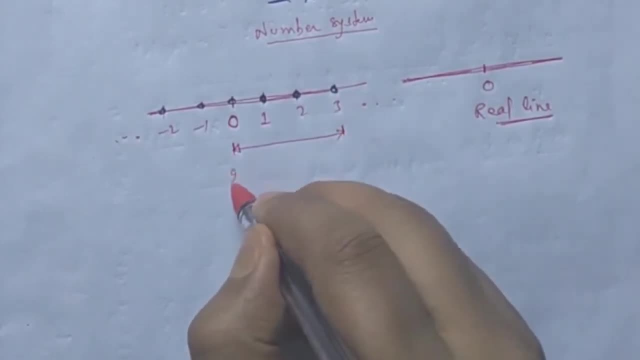 between 0 and 3. so here we have plotted integers. so if we have plotted integers and someone asks that how many numbers are there between 0 and 3, or if we have to count this too, then we can say that 0 to 3. 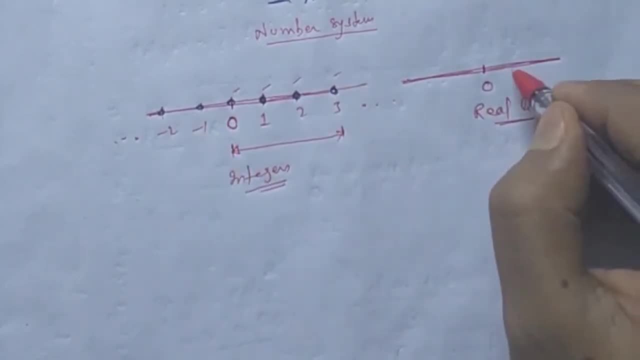 we have 4 integers in the complete part. but if this case we have real number on the real line. so if we have plotted the real number, same case. and here, if someone tells us that, tell me how many numbers are between 0 to 3. so can we say here: 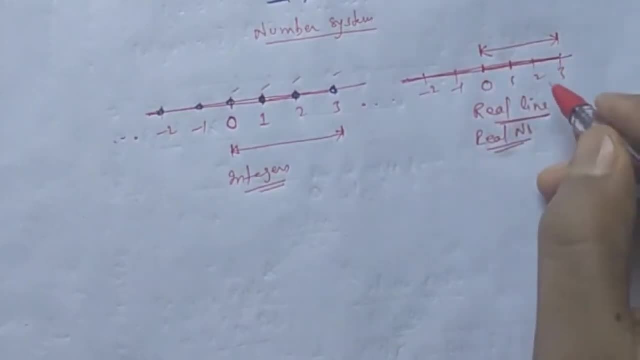 how many numbers are? between 0 to 3, there are infinitely many numbers. infinitely many numbers means we will not be able to count it and in the case of real number, if we choose any two numbers in any interval, then there are so many numbers in between. 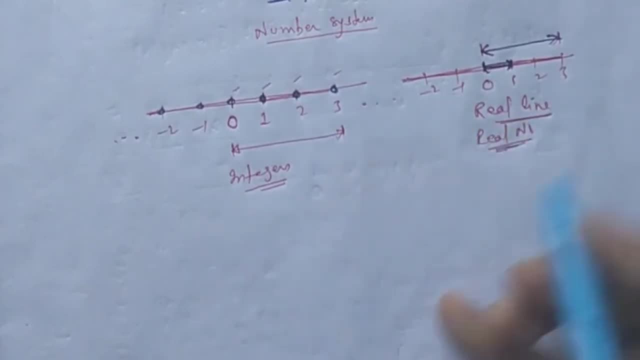 that it cannot be counted, but in the case of integer, we can count it. so you must be understanding these two things. we are dividing the system into two parts. one is called discrete system, right, and one is called continuous system. so this is continuous system and this is discrete system. 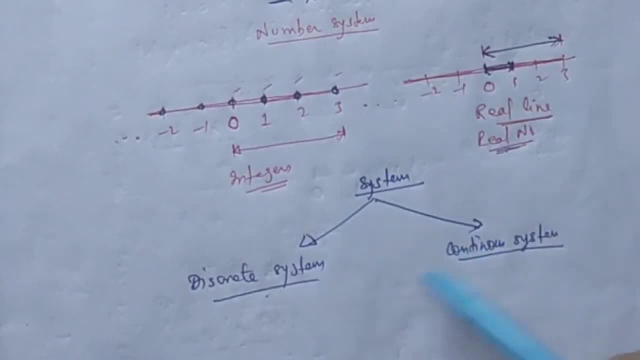 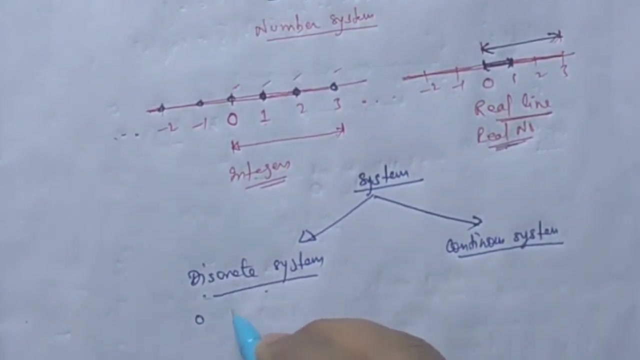 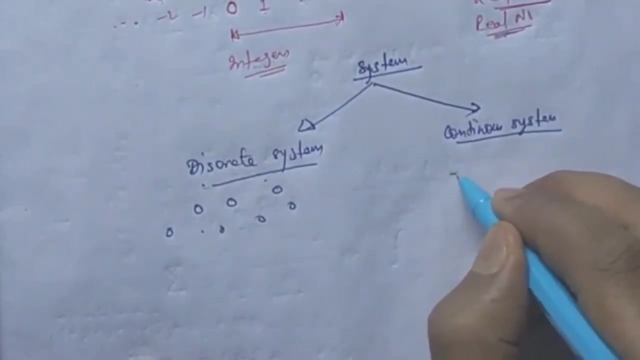 if we divide these two things on the basis of this parameter, then what will be the integer? it will be discrete system. you will see something like this. and how will be the continuous system? you will see something like this here. you will not be able to differentiate between two elements. 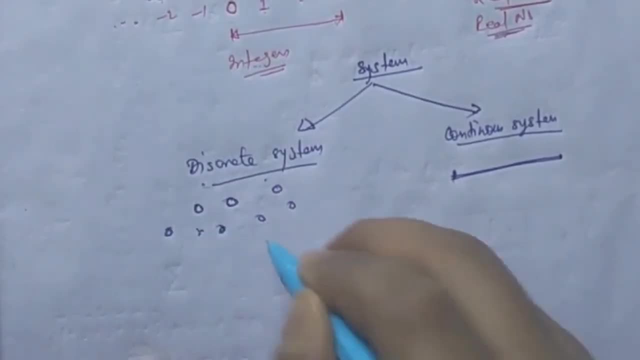 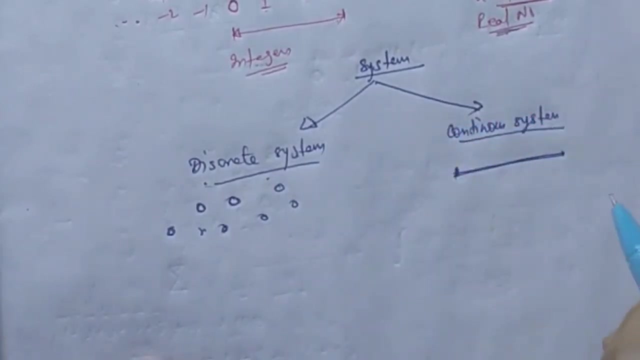 but here we are seeing different elements. right so, on the basis of this parameter, we are defining our system right now. if we try to understand this through example, right so when you go to the market and you want to buy milk, right so what do you say to him? 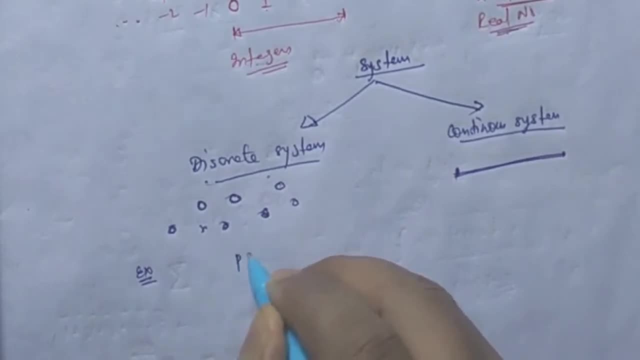 that I want milk packets, right? so if we buy milk packets, then what are these milk packets? it will come in discrete system, how that you can buy number of milk packets. you can buy 5,, 10,, 15,, 20, whatever, but you can buy a countable number of milk packets. 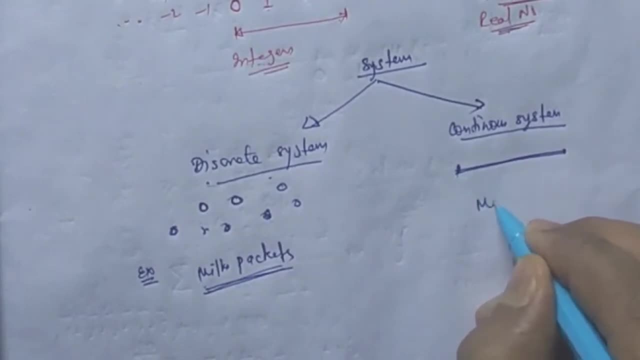 but the milk inside the packets? can we call it discrete? we can not say: right, we can see the packets separately, but the material inside the milk, the material inside the packets, the milk, we will never see it separately. what is that? it is a continuous system, right? so milk is a continuous system in itself. 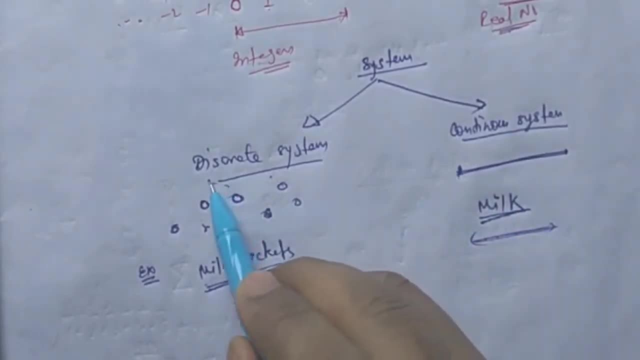 so in this way we are understanding through the example, that discrete system and continuous system can be of which type right. so when we have to add discrete system, then what do we use? there we use sigma right. and when we have to add continuous system, then what will we use? 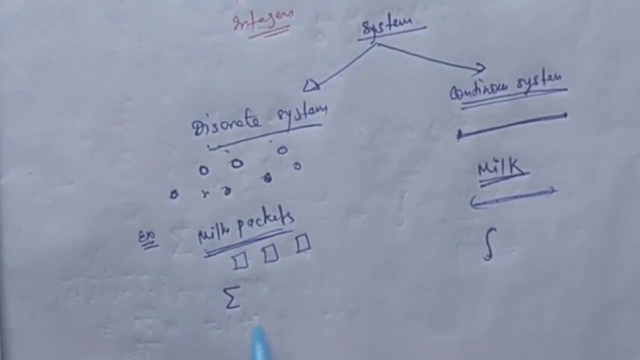 we will use integration clear. so these are the two types of difference: where to use sigma and where to use integration. both work. we have to do sum, but both sum can be used at different places. we can not use it here. we can not use it here, right? 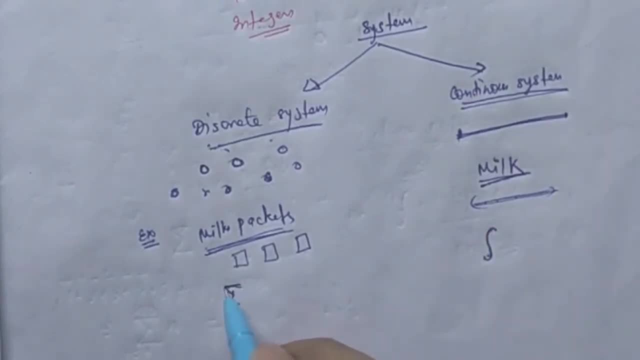 so this is the basic difference in both. now, how does this sigma work once we understand it? this part we will in physics, in basic maths. we will complete it right, the basic maths part which will come in physics and which we are saying mathematical tools, right? so in this mathematical tools part, 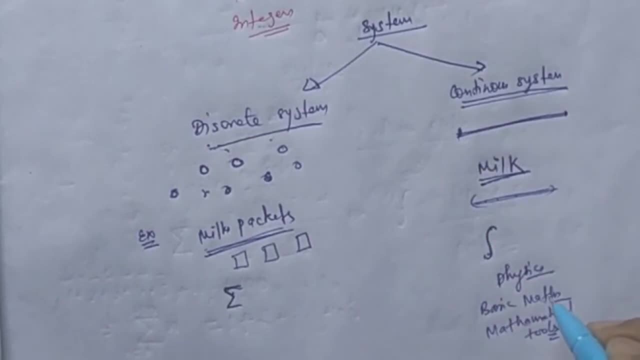 you these things will be clear in a better way. the integration part: how we are using this symbol and adding in this part in maths. for now, we will see this sigma part, how this sigma works. you have already seen this in tenth right. once we will revise it. 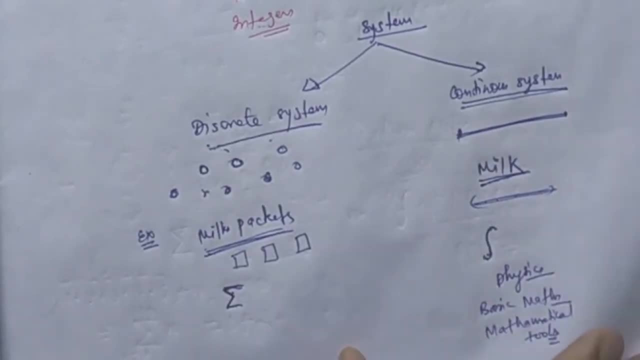 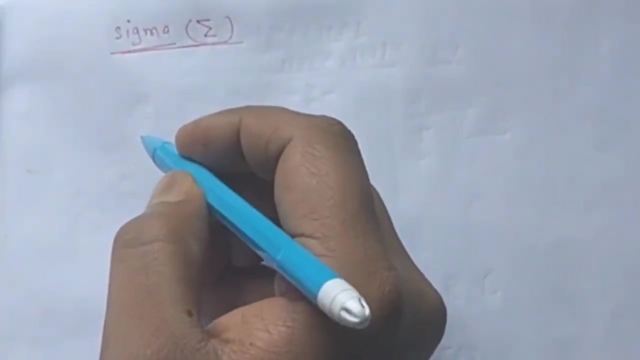 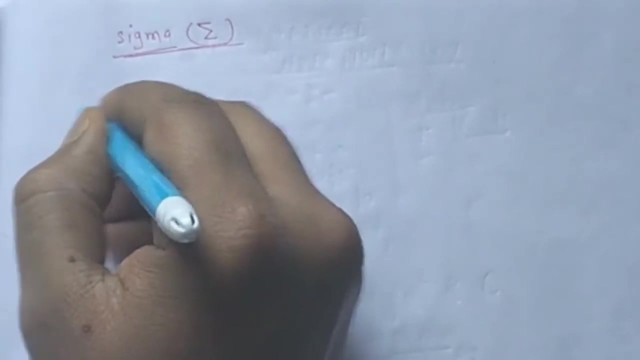 right. so next we will see how sigma is working- right. so now we are seeing what are the things in sigma notation and how it works. so we will see this first. that suppose we have to write this sum from 1 to 3 if we have to write 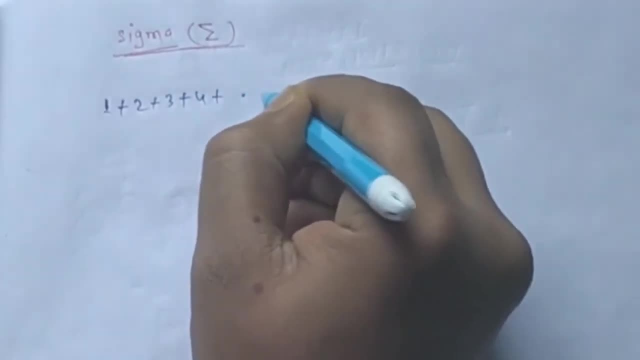 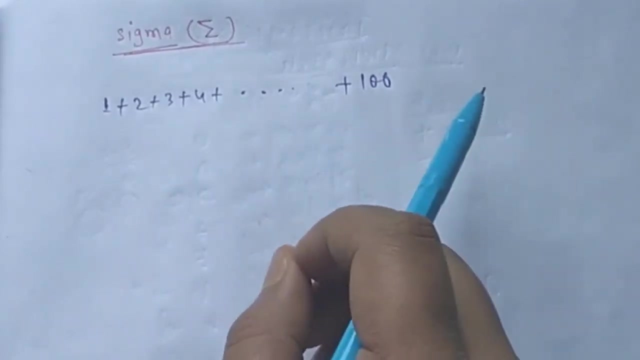 the sum of all numbers till 100. right then, how can we reduce this sum in simple notation, right? so this type of notation, this lengthy notation, to reduce it we use sigma symbol. right, so see here, if we write this sigma symbol. right? so see here, if we understand this. 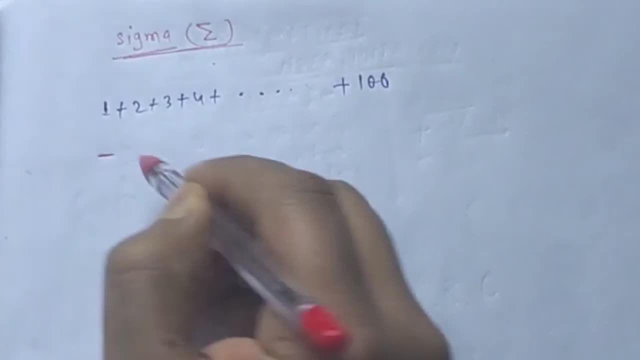 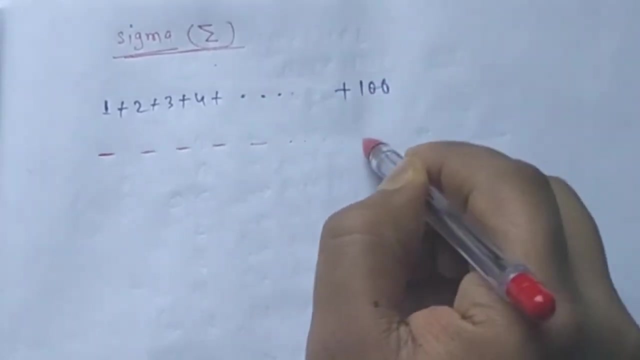 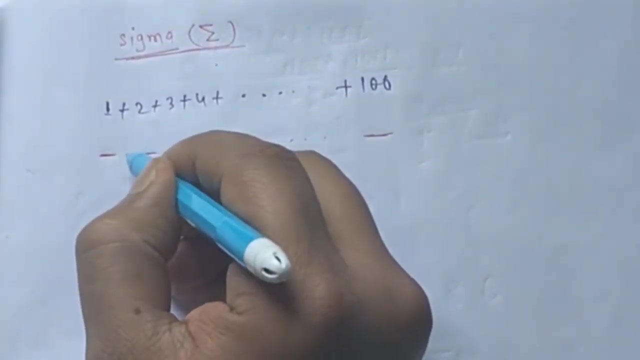 in a better way. so here we are denoting this one as a dash right. so here, how many dashes: we have 100 dashes, right? you must be understanding these things, because we have 100 numbers and between these 100 numbers what we have. notation of plus symbol. 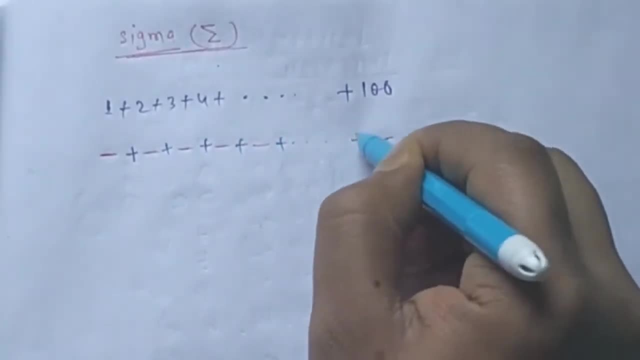 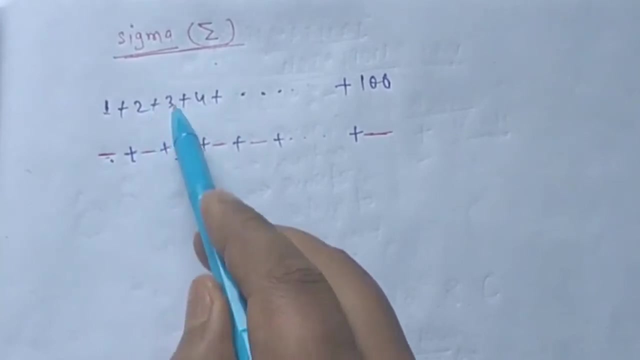 right. so in all this, a sign of plus is coming from this type. so we have two types of notation. one is a dash where we have to fill number right and sign of plus- now see these things are happening repeatedly- just the place where we have to fill. 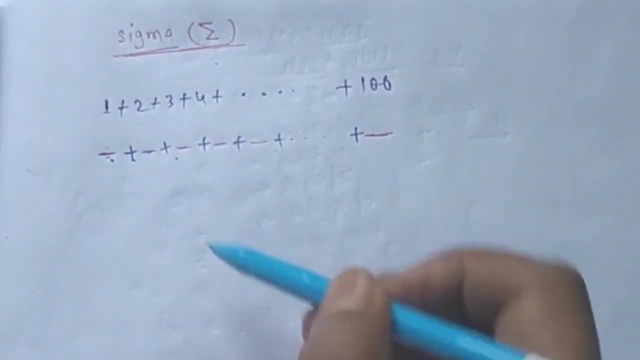 we have to fill number. but this position is fixed, right? so if we write it in simplified version, so actually what we have one dash and one plus symbol. so we have dash plus symbol, right? so just on the basis of these two notation we can generate this thing. 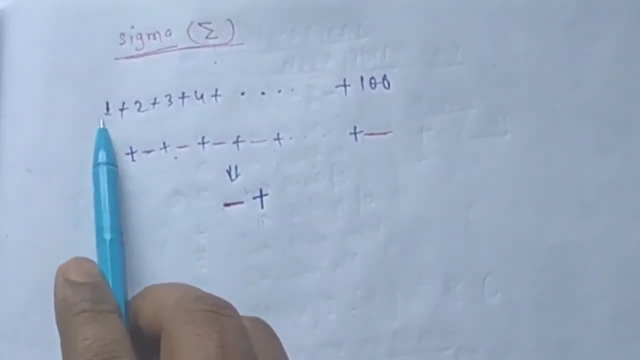 just this blank space. in this space we have to one, two, three, again and again different terms have to enter, right? so we can understand it in this way that actually how it will work like a variable variable. who is saying that? who is changing its value? right? so if we 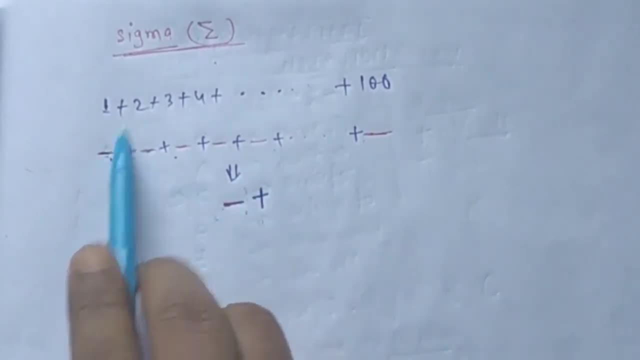 put a variable right so we can represent these things in this way right now. if we say that, suppose we put n here. now what is n? so we are saying n here, variable right, what does variable mean? variable means that which is changing its value repeatedly. so now, 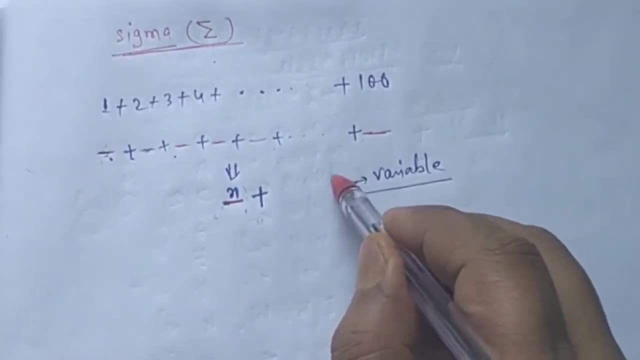 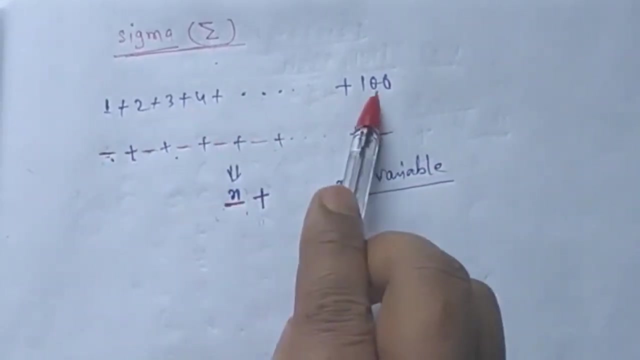 we have said n as variable. so first of all someone will ask us that what is n? so what value is he taking? so what will we tell him? that value of n- one, two, three- may be from four to hundred, meaning how much value is taking n? it is taking hundred. 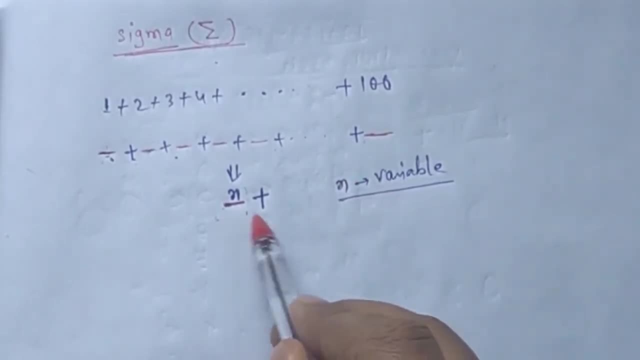 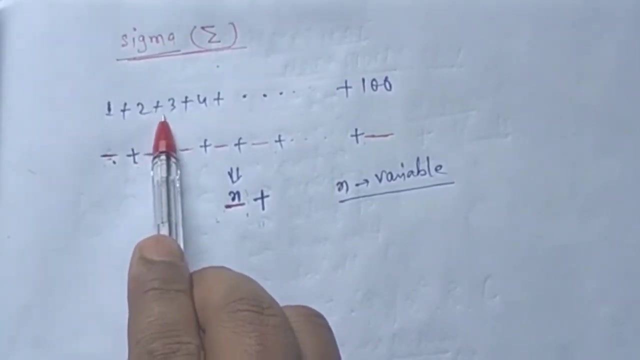 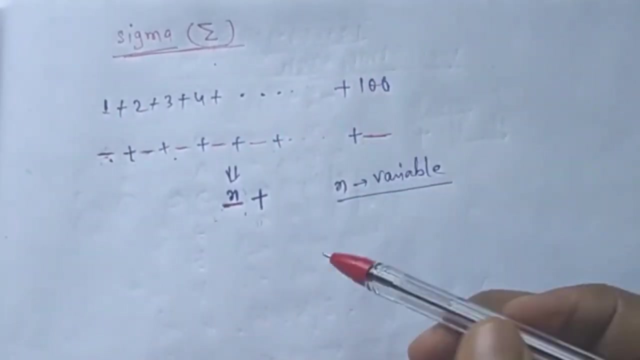 right. so we will put n value according to us, right. so if we use this symbol, first of all will put n value one, so here will be generated one, and then is a plus sign. we can generate this type of expression by putting different values. so on this basis, we want to write it in the form of symbol. 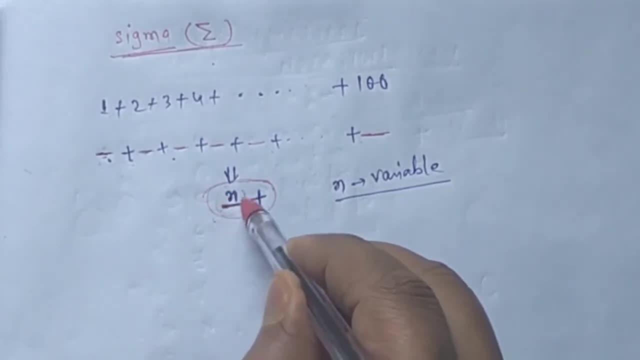 first of all, we understand that we need a variable. so we are introducing a variable first and the value of n will go from 1 to 100. so in our mind we know that this is a variable n and it is taking the value from 1 to 100. 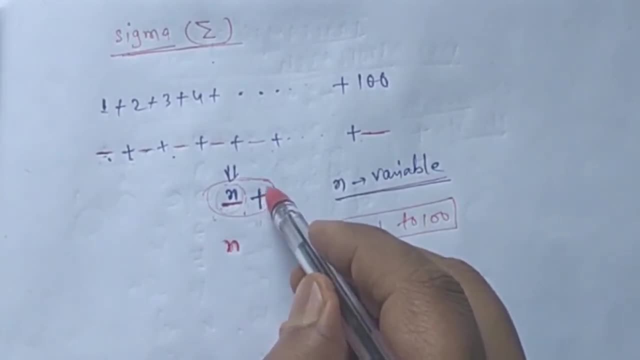 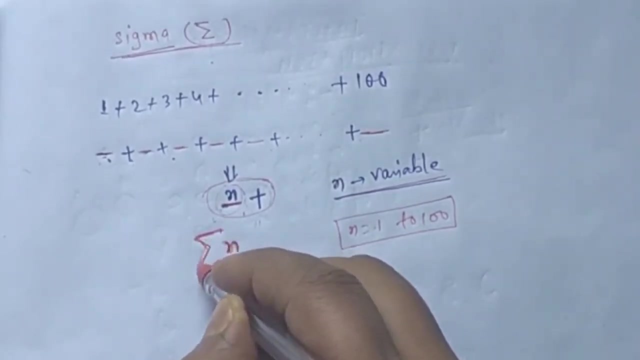 now how we will replace this plus symbol. for this plus symbol, which term is coming here? Sigma. so if we want to replace this notation, first of all we have to put a sigma sign. what is this sigma symbol we have to add, to which we have to add: 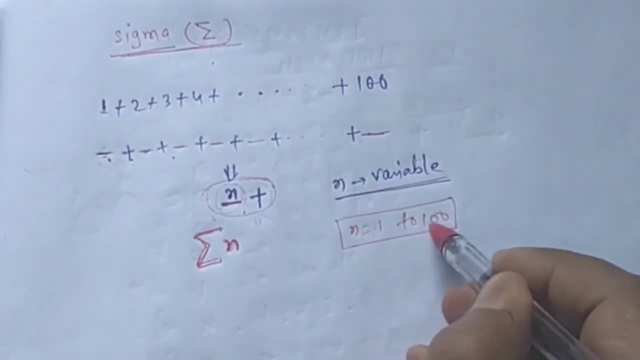 n and from where to where. we have to add n from 1 to 100. so we know the value of n from 1 to 100 and we know this. but if someone reads this expression, then how will he know that we have to add from 1 to 100? 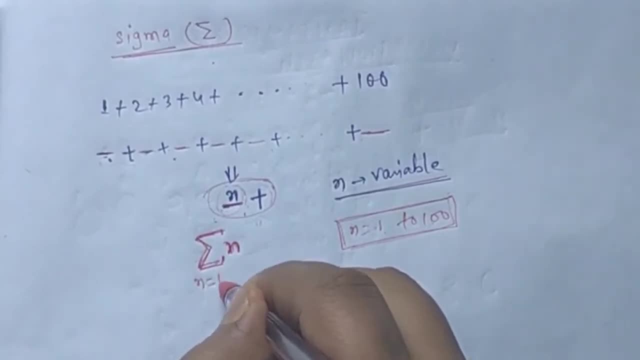 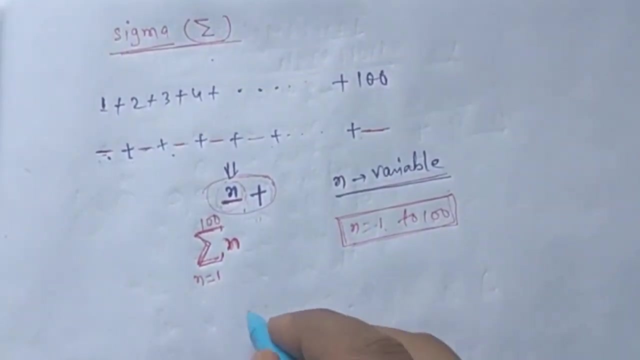 so what will he do? here we have to write n equal to 1 to 100, and what do we call this? and if we write it in a good way, then first of all it will be a sigma symbol. after that we have here we are writing, an expression. 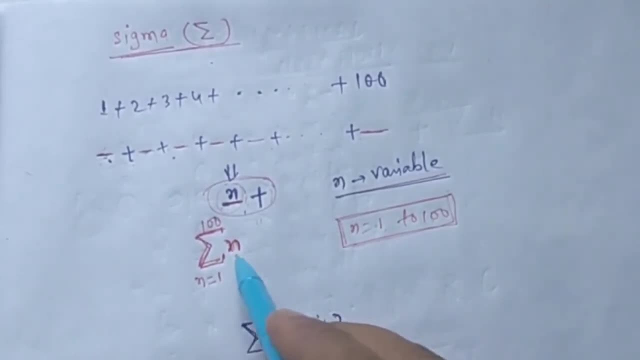 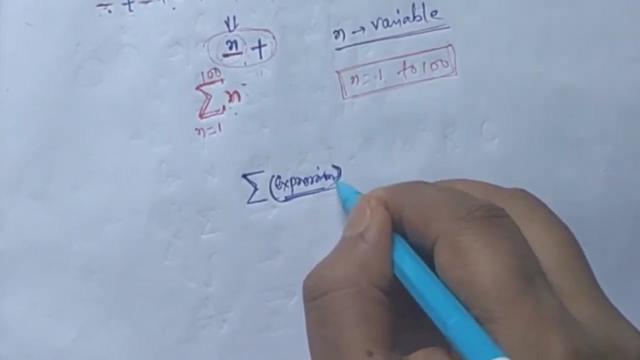 what will be the expression in this case? what was the expression? we had n, but this expression can be of any type. here we have changed it, so we wrote n, so here we are calling it expression and here we are writing the variable in this expression. so whose expression will it be? 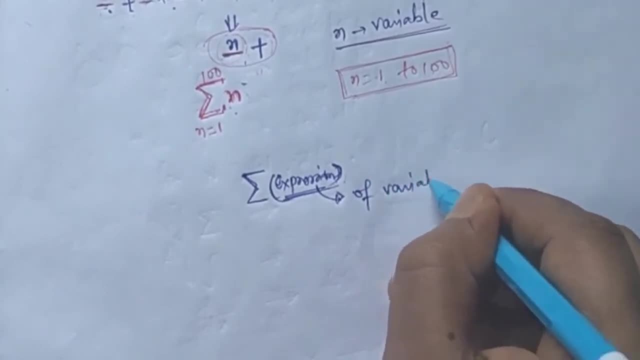 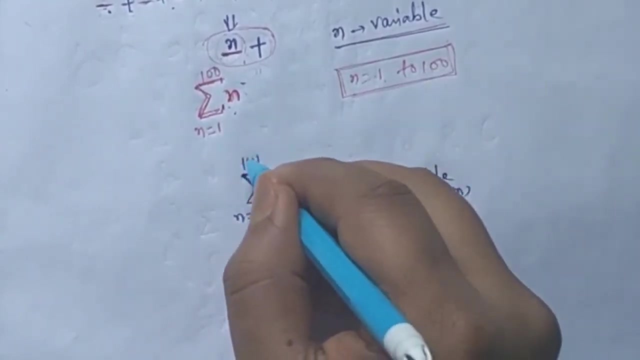 of variable. so now we will see some examples where this thing will be clear. and here we have the value of this variable. let's say we are calling this variable n, so the value of this variable n equal to 1 to 100. for this case we are calling it. 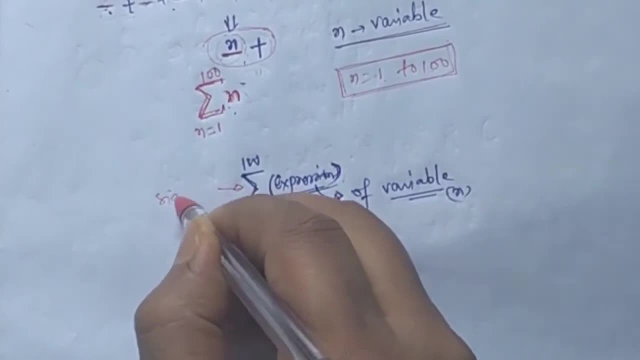 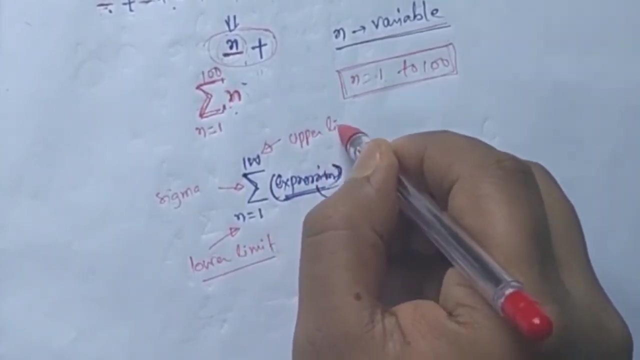 so here we are seeing. what is this symbol, what we are calling this lower limit. we have to see where our variable is starting and what we are calling this upper limit. so how far will it go? ok, so we have to pay attention to these three things. what will sigma do? 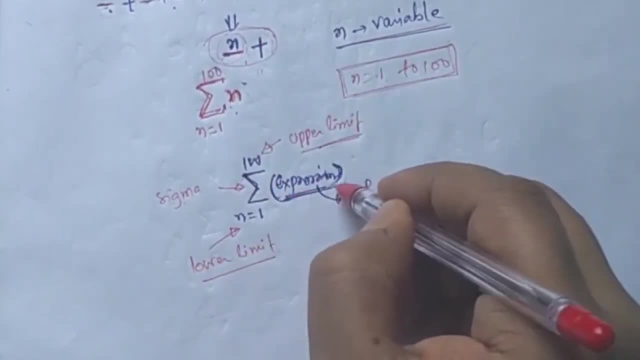 it will generate the sign of plus again and again and in this expression the variable. this is the lower limit of that variable and this is the upper limit. and when the value of n is 1, so how much will be the value of n next time? so we have to do the increment of 1 to 1. 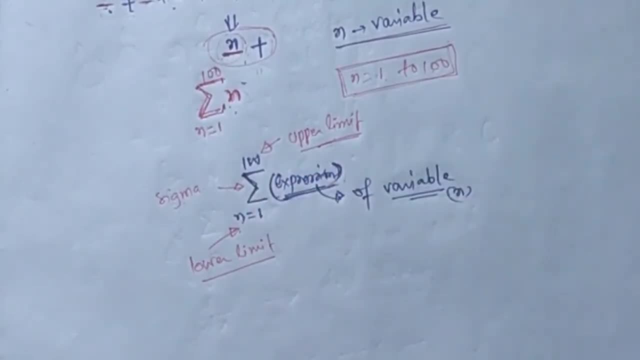 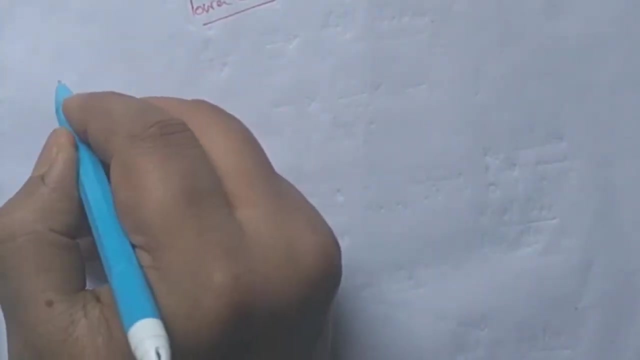 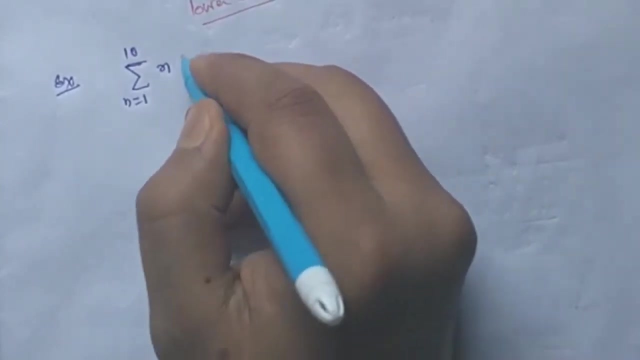 right. so now we understand this through example. that suppose we have one expression of this type. ok, if we have, this is sigma, sigma equal to sigma, n equal to 1 to 10, and here we have taken n, and if we have to open it, we know that it is written in symbolic form. 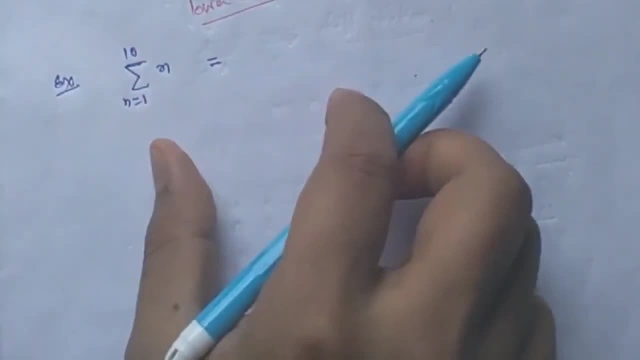 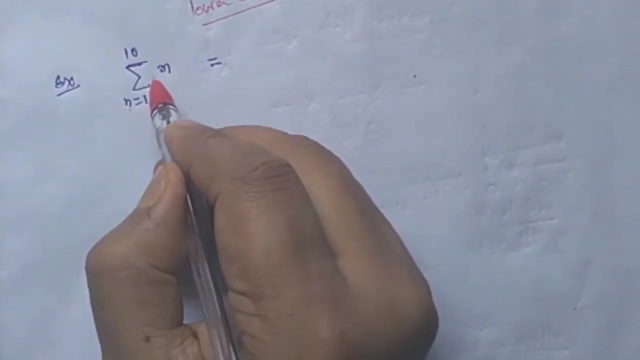 but if we have to open it and see how it is working. so, first of all, what is the variable we have? so here you can see that this expression, the expression we have taken here, this is the same expression. so here the expression is only n and the variable is also. 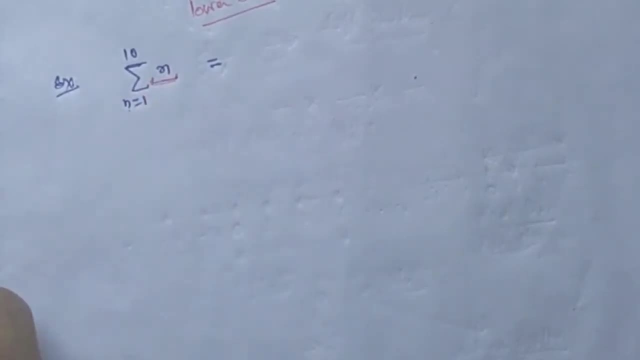 n only. so what? we have to put the value of n first. we have to put 1 because the lower limit is starting from 1. so this is 1. after this, this is the sign of sigma. so for sigma we will give the sign of 1 plus. 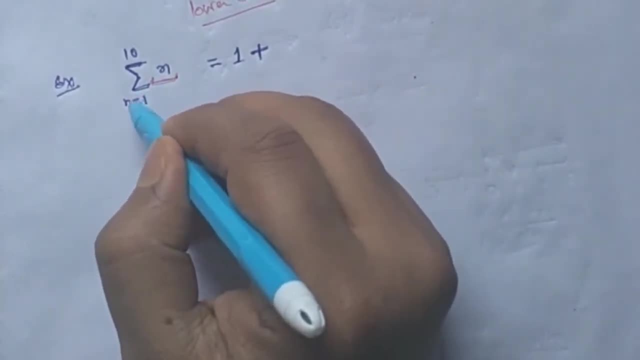 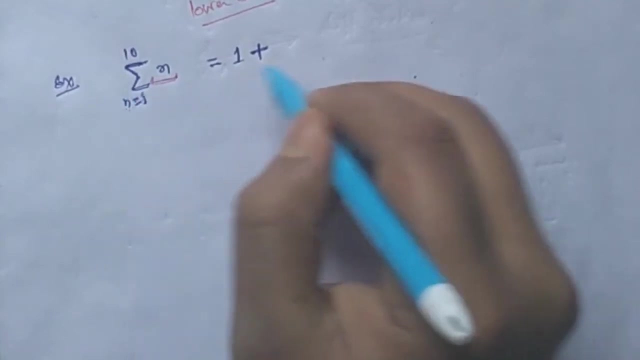 and after this we have to know the value of n. we have to go till 10. but to go till 10 we have 9 digits in between, so we have to go to all of them. so after n equal to 1, the value of n will be 2. 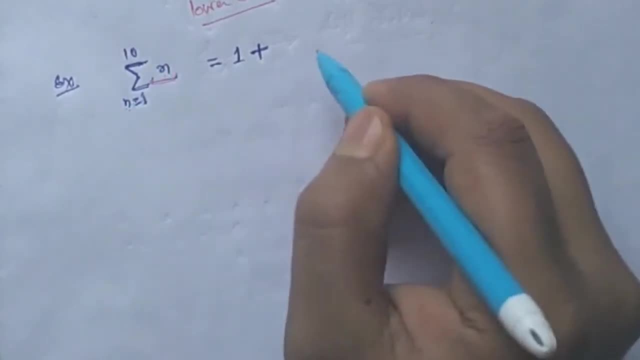 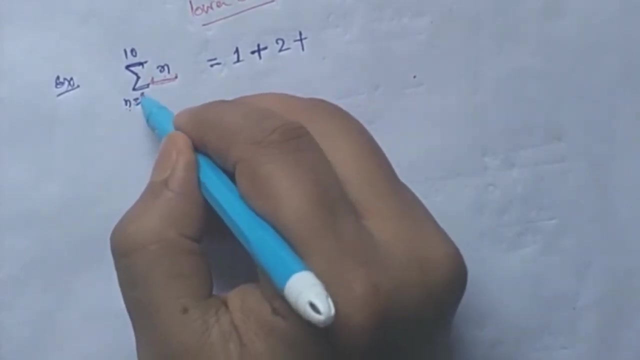 so we will put the value of n 2. so in this expression we will put 2 instead of n. so here we have put 2 again. this is the sign of sigma. so what will this sign do? it will give plus symbol. then how much will be the value of n? 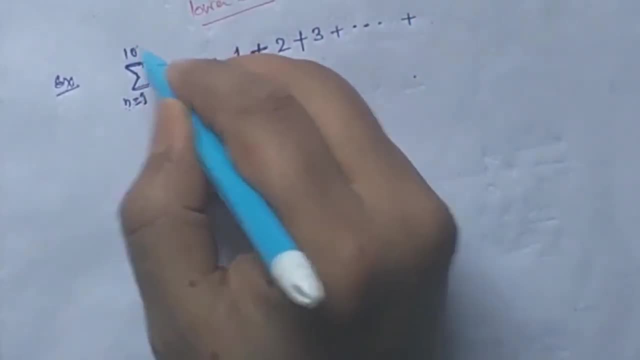 it will be 1 increment, so after 2, next 3, and in the same way this symbol will go till 10. is it clear? next, if we try to understand from another example, we have to know the value of n from 1 to 5. 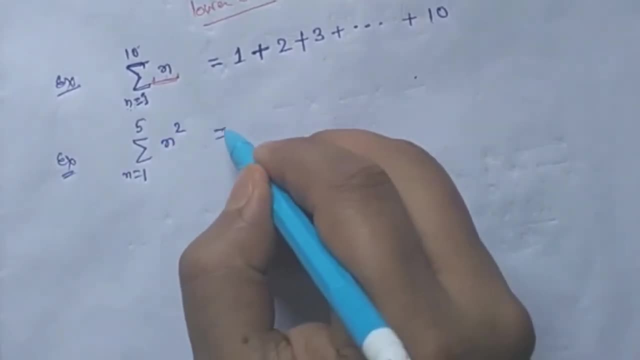 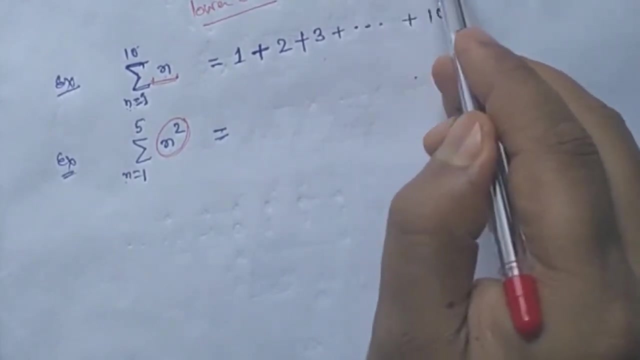 so if we open this, what will we get? so let's see what is the expression. so here we have this expression: n- square, and what is the variable? variable is n. so here you can understand what is the meaning of expression and what is the meaning of variable. 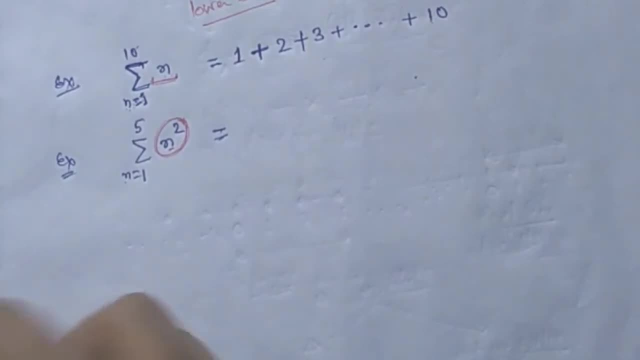 so first of all, in the expression we will put the value of n. so if we put the value of n, then what will be the value of expression? 1 square, and this is the sign of sigma. so here we are using plus symbol. similarly again in n. 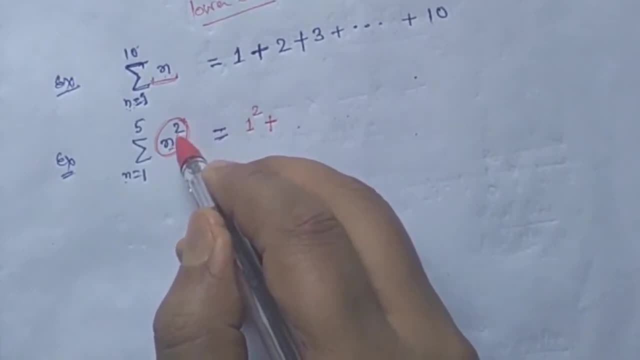 what will be the value of 1? so in this expression we will put 2 instead of n. so what will be the value of 2? again the sign of sigma, plus again the value of n will be one increment. so what will be the value of this symbol? 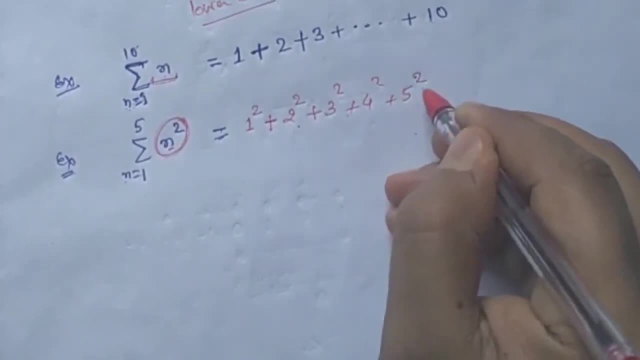 3 square and when we write it completely we have to go till 5 square. the value of n should be 5 and this expression is creating 5 square. so this many times we have written this expression in the form of a symbol. now you can understand. 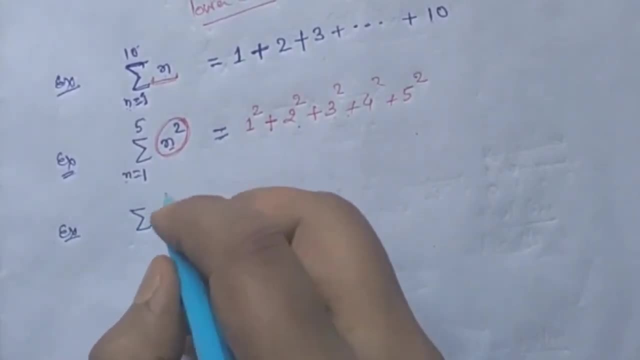 what type of question we are talking about. let's take one more expression twice: n plus 3, n equal to 1 to 10. let's put it again now. see here: expression is this complete expression? whatever term is written with sigma, that will be complete expression. 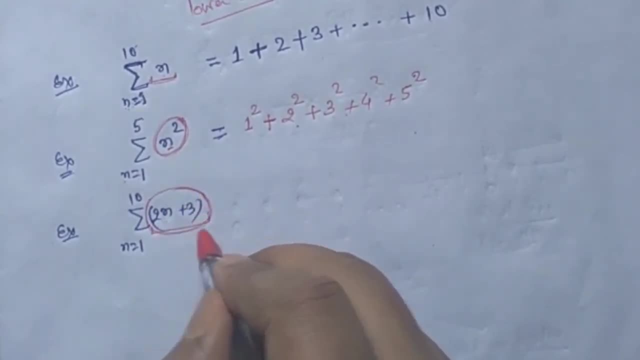 is it clear. and in this expression, what is the variable? variable is n, and again we have to go from 1 to 10. so again, what will we do? we will put n equal to 1 when we will put n equal to 1 in this expression. 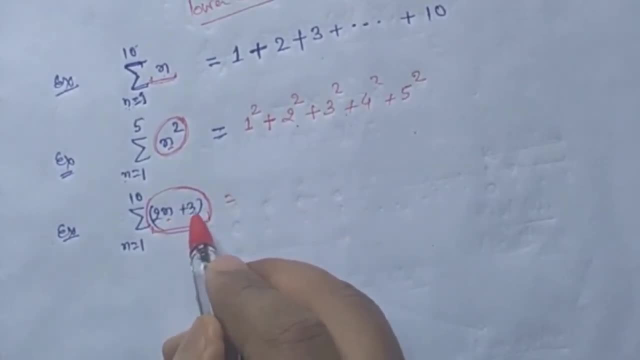 then see what will be the value: 2 into 1 plus 3. what will be the value of this complete expression: 5? isn't it again the sign of sigma? so we have put plus. then we will do one more increment in n, so it will be 2. 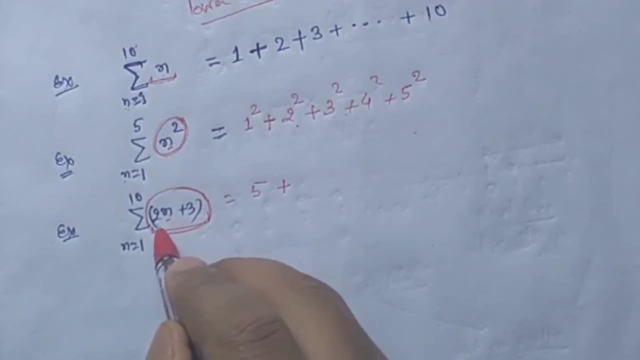 in this expression we have to put n equal to 2. when we will put n equal to 2, then how much it will give. 2 into 2 plus 3, 7, again the sign of plus. we will put n equal to 3, then how much it will give. 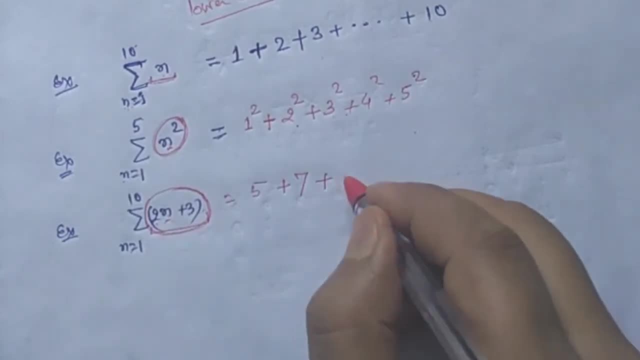 2 into 3 plus 3, 6 plus 3- 9. is it clear what will be the next term when we will put n equal to 4, 2 into 4 plus 3, and how much will be the last term for the last term? 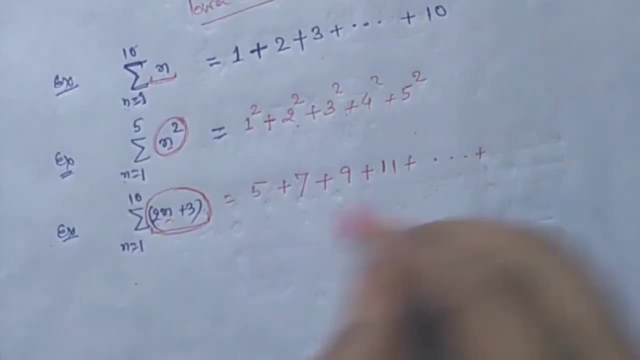 we will put the upper limit- so how much it will be? 2 into 10 plus 3, 23, isn't it? so sigma works with this type, isn't it? after this, so you must be understanding these things. now we will see that some properties are there. 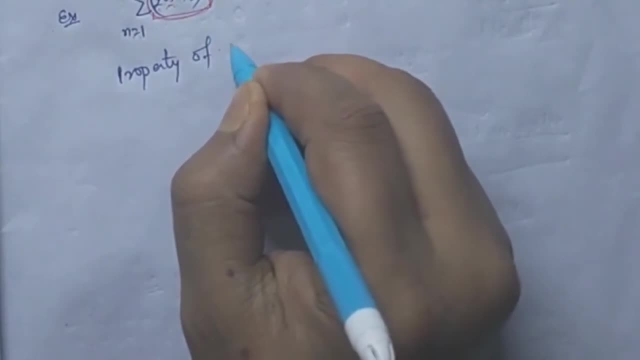 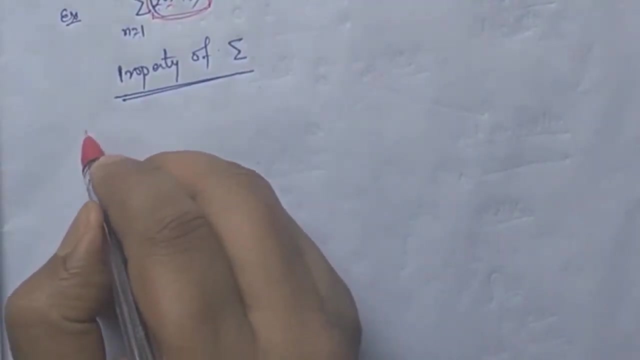 so we will understand that property, property of sigma. ok, so, in property of sigma, the first thing is that we have sigma. if we have two functions and two types of expression, one expression is of f of n and the other expression is of g of n, isn't it? 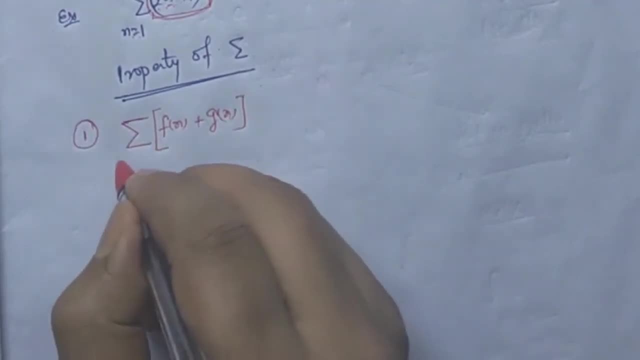 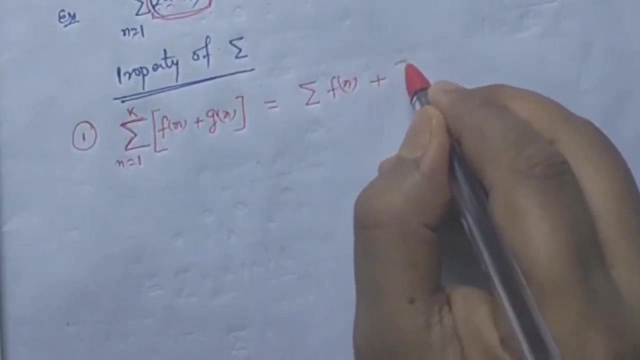 so if two types of expression are in the form of summation, and here n is moving from 1 to k, so what we can do with this expression with sigma, we can break it separately, isn't it? so we can break it in f of n plus sigma. 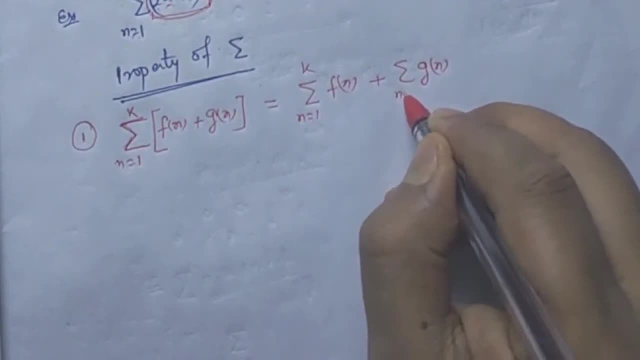 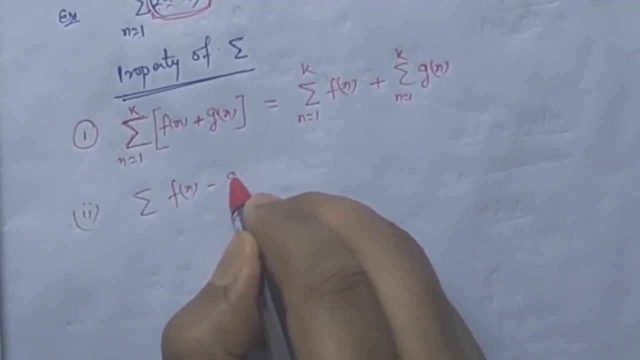 g of n, n equal to 1, to k rest. there will be no changes. we just break it separately from this part. so in case of sigma, these things are valid, isn't it so? if this type is with minus, isn't it so what we will do in minus? 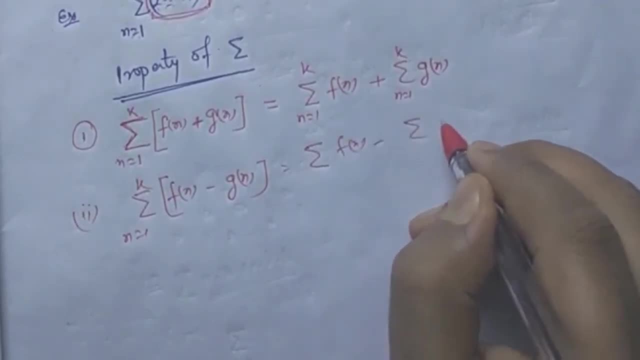 these things are in minus. we will break it separately: f of n minus sigma g of n. n equal to 1 to k. n equal to 1 to k, isn't it? and third type of expression: if in any expression any constant is being multiplied, this is a constant. 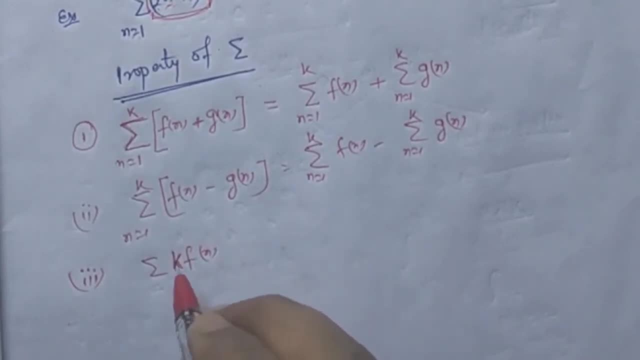 isn't it? what is a constant whose value will never change? for example, 2 here, 2 multiplied, 3 multiplied, 100 multiplied, isn't it? so? this is not depending on n. there will be no difference between n and k. n equal to 1 to k. 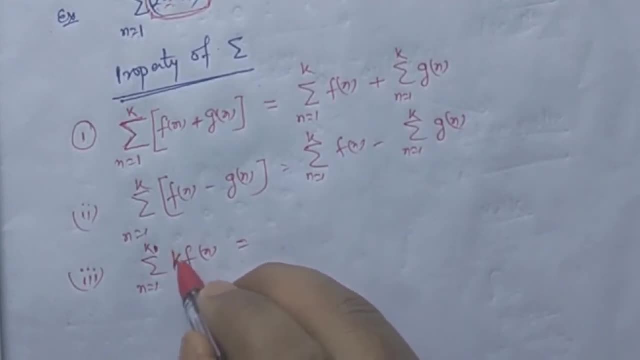 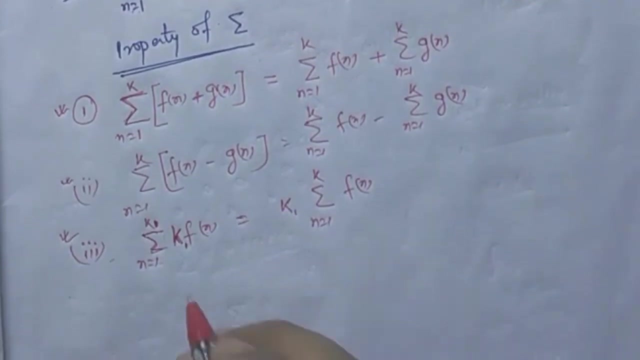 isn't it. and take this as k1. this is k1, and take this as k2. along with that, we can take this out of sigma, isn't it why? because this n value has no difference from this. n equal to 1 to k. f of n. 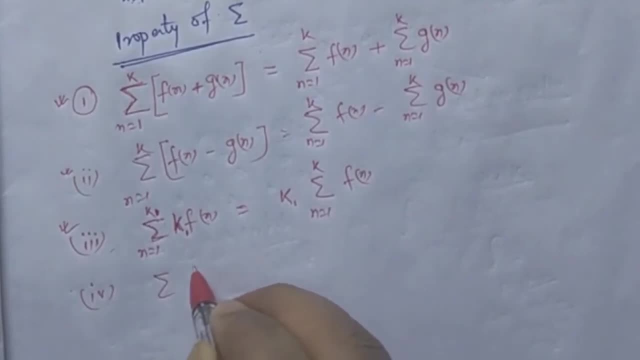 so these are 3 important property. we have to keep these. after that, fourth property, if we have, we are moving. so in different functions we will be able to multiply sigma by doing it or not, As we did in addition and subtraction. so we solved both separately and multiplied. 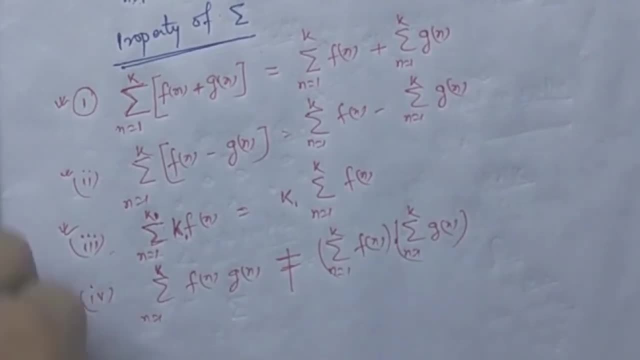 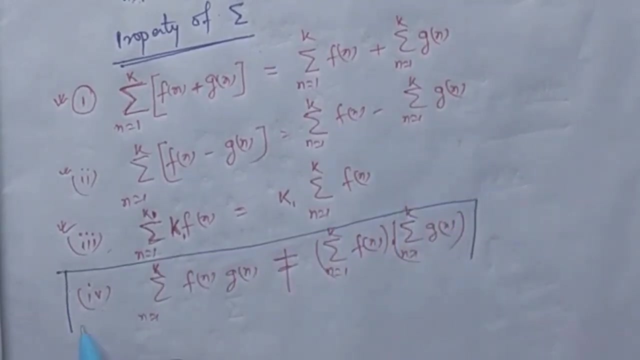 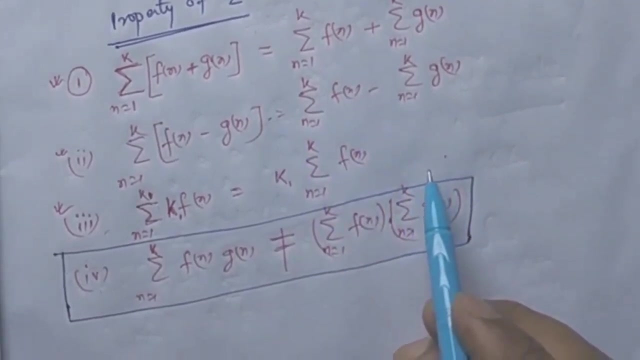 both separately. So these things are never valid, okay, that's why this point is written, because the maximum error is here, because we know the rule of addition and subtraction, that it is different. so what do we do, students? that we apply the same rule in this too, so we do not have 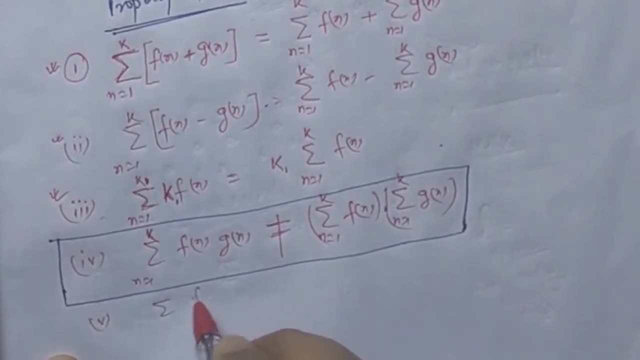 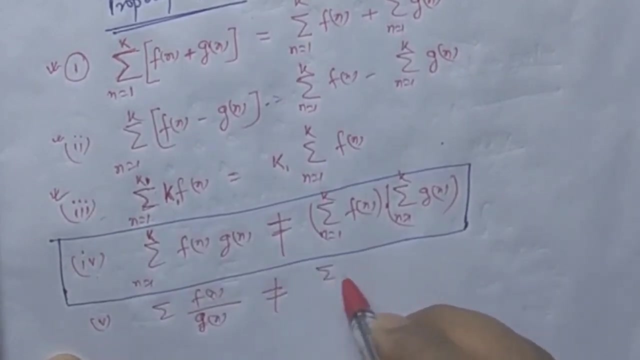 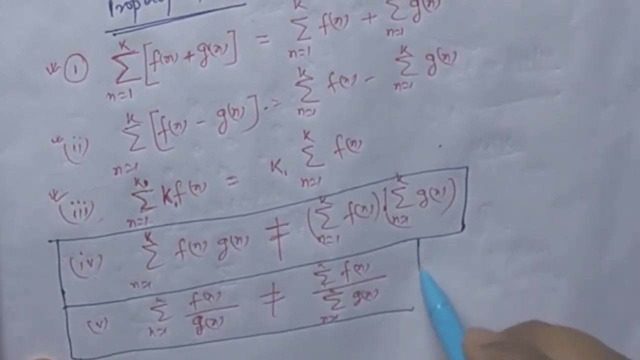 to make this mistake. and the same rule is also valid in the case of division. so if we have sigma in division, then we will not be able to break sigma separately in division either. So these two rules are very important, right, we should know this thing, but at the same, 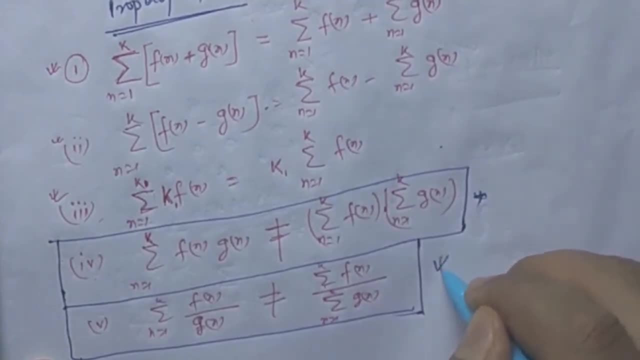 time. we should also know that we do not have to make these two mistakes. so we have five rules. we can apply three rules out of five rules. we do not have to apply two rules. so we have to take care of what we do not have to do. 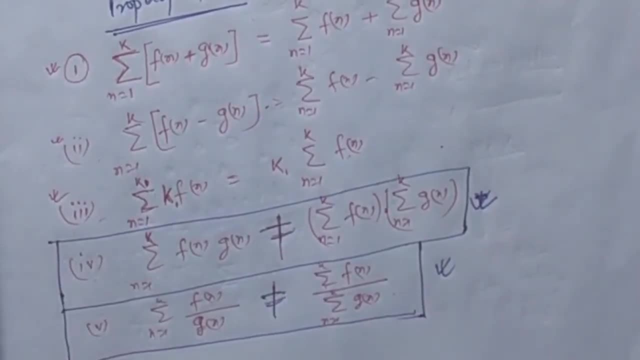 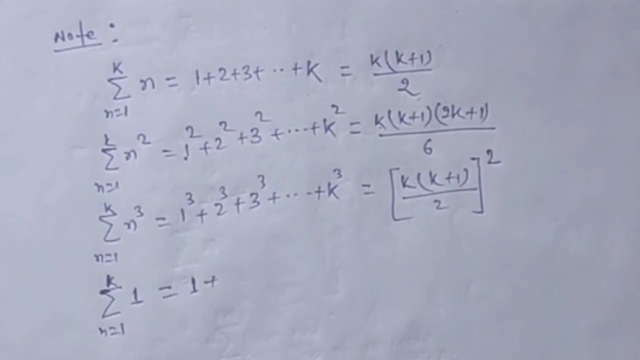 Okay, so we have to do it. you need to have this rule. you have to do it. the rule is very important. okay, so now we have seen that how sigma works. if it is in addition or subtraction, then we can break sigma separately, but in multiplication and division sigma does. 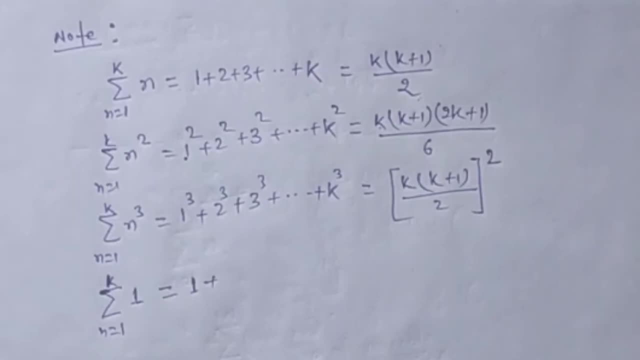 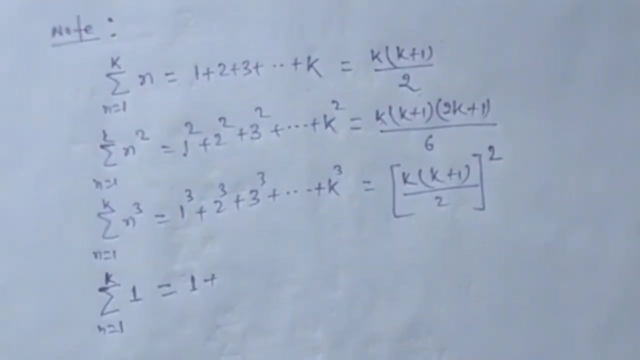 not break separately. so we always have to keep these things in mind. Now let's come to some particular type of specific sigma notation, right? so we have to keep this thing in mind a little bit. Okay, we are going to use these things again and again. 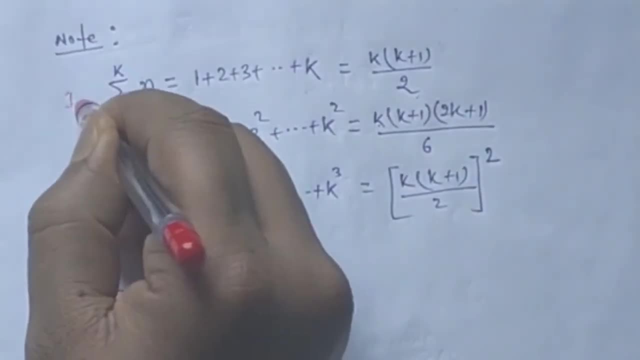 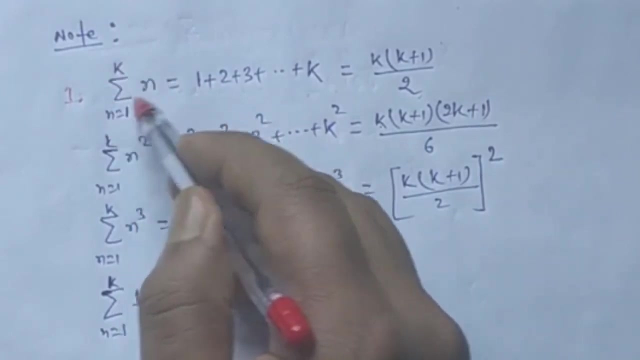 so, like the first one is sigma n. when we put the value of n as 1, then this expression will give 1, and we know how to expand this sigma notation. so if we expand it then it will go upto 1,2,3, upto k. 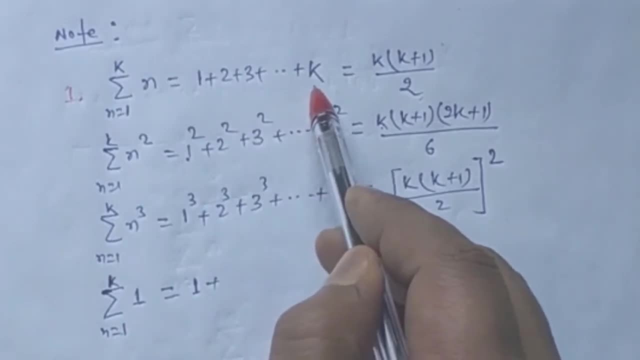 because the upper limit is upto k and if we have to write the sum of this, then we can directly use this formula. so if we have to write the sum of 1 to 100, then directly put 100 instead of k and your answer will come out. 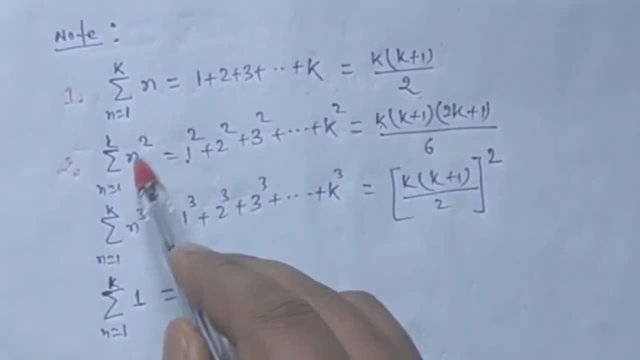 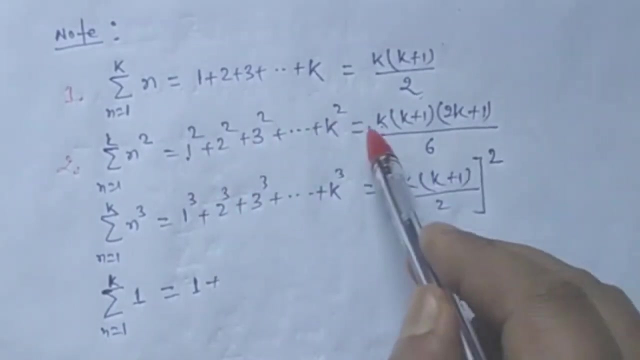 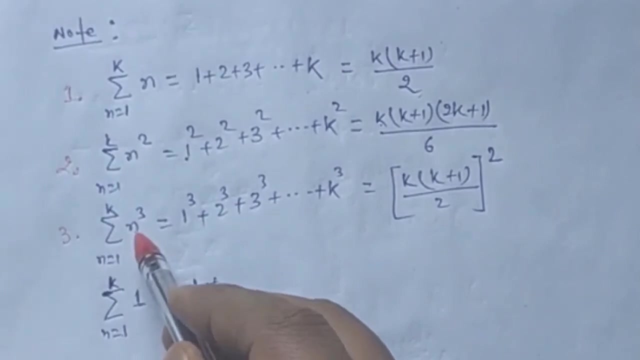 similarly, if we have the sum of the first natural number of sqrt, so 1 sqrt, 2 sqrt upto k sqrt, so if we sum this, then what is the value of this? it comes from this type and the third type is sigma n cube. and how will we calculate the value of n cube? 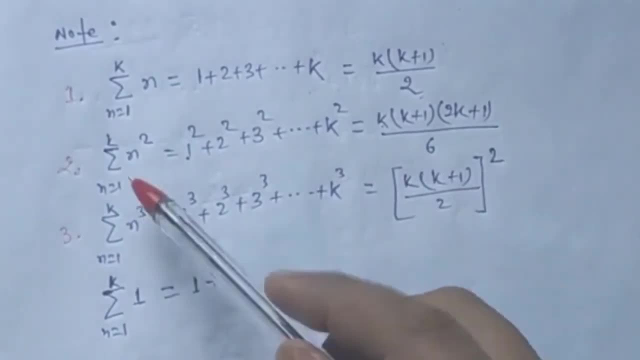 if we expand it. and what is the formula of this? see here: the formula of sigma n is equal to sqrt. so you should remember these three formulas, all these in detail. there is proof that how this thing comes out we will see in the sequence series. similarly, there is a fourth type. 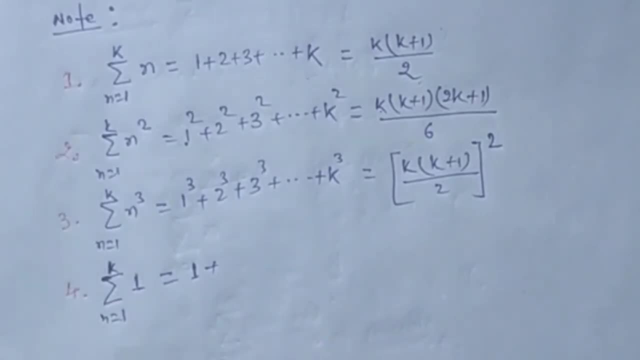 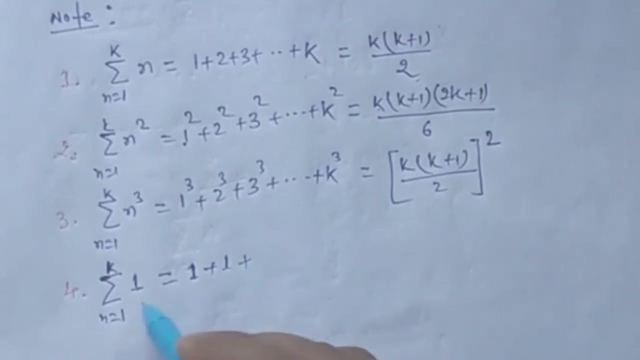 where we are writing sigma 1. what does sigma 1 mean? that this expression is not independent. so if we put the value of n, then how much expression we will get? we will get 1. when the value of n is 2, then also we will get 1. 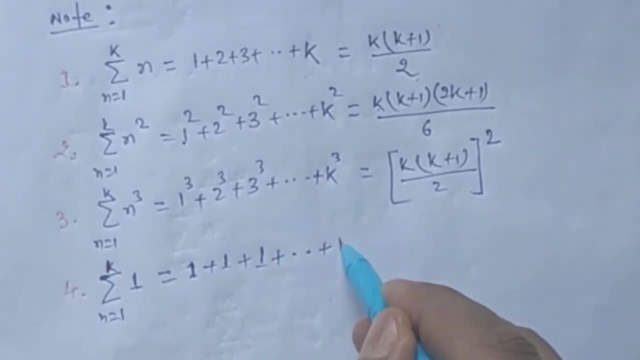 when the value of n is 3, then also we will get 1, and till when we will get this till the value of n is k. so how many times is this repeated? now you must be understanding how many times is this repeated k times. so these are the four formulas. 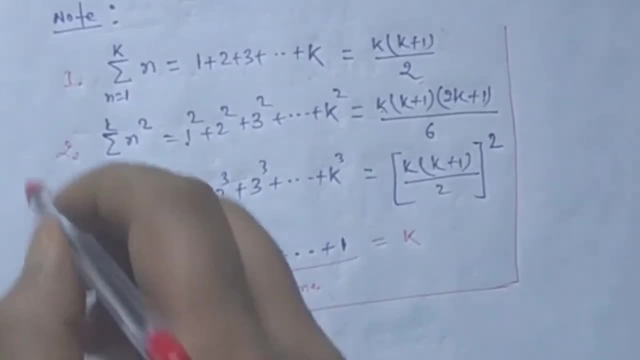 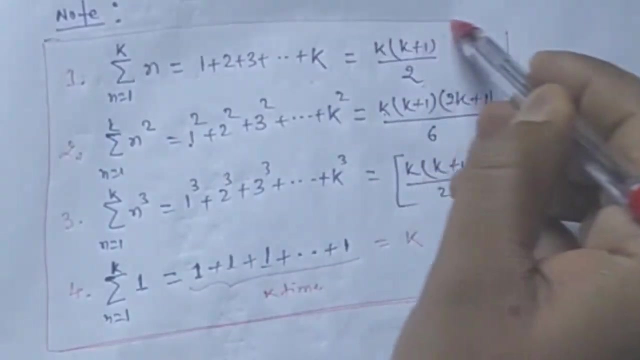 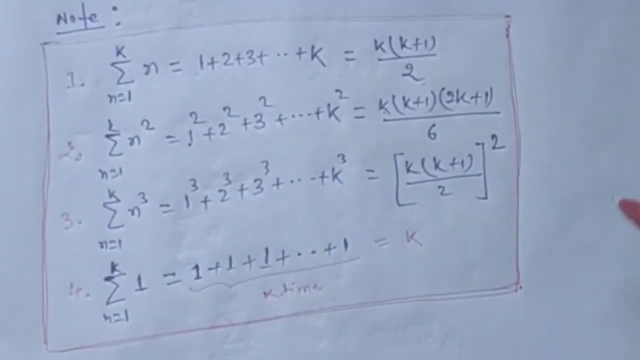 these four formulas. we should be paying attention to these four formulas. if you are not able to remember now, then no problem, but these things you will understand automatically and these things are repeated so many times that you do not have to remember. we understand these things through questions. 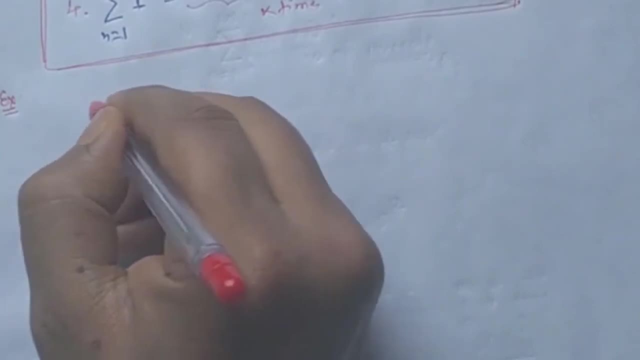 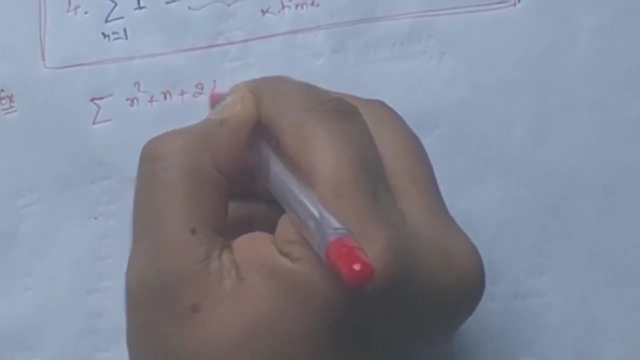 now we will see some examples on sigma notation, like if we have n square plus n plus 2, and here we are adding n value from 1 to 10, and here we are adding n value from 1 to 10, and here we are adding: 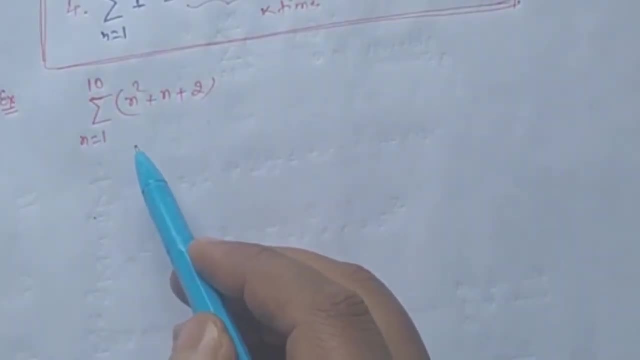 n value from 1 to 10. so how will we calculate this expression? so here we can see that the expression with sigma is in the form of sum, and just now we saw that we can break the sum of sigma separately in this way: in 3 sigma. 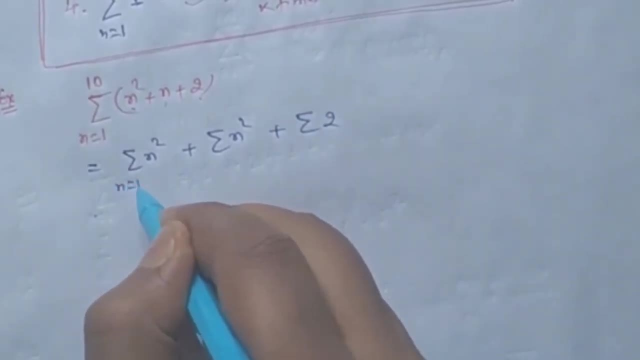 you are understanding, and there will be no changes in the lower limit and upper limit of sigma. there is n here and this is n equal to 1 to 10 and this is n equal to 1 to 10. now see how much we will write. 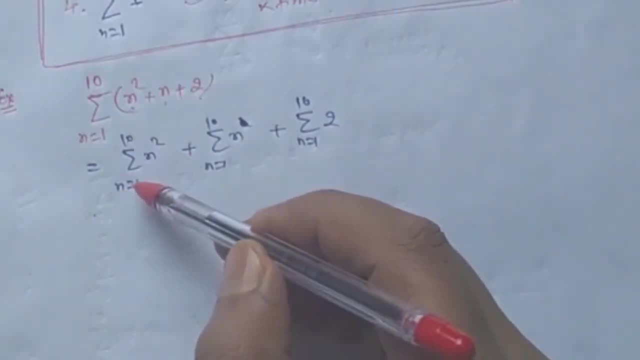 sigma n square. so just now we have seen the sum of sigma n square. we just have to see the upper limit and in that formula we have to put 10 instead of k. so the answer will be 10 into 10 plus 1 into 2, 10 plus 1. 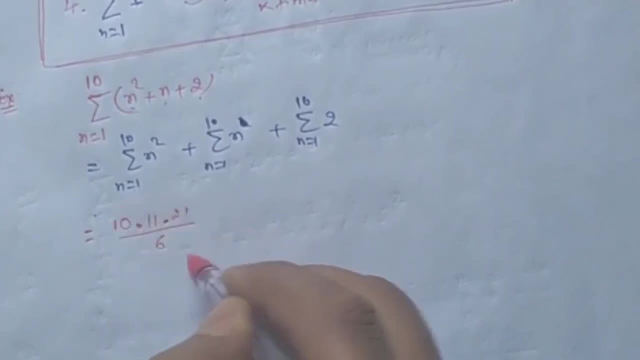 divided by 6, we can solve this expression. we can solve this expression plus sigma n. what will be the value of sigma n? see in the formula. simply, we have to put the value 10 into 11 by 2, 10 into 11 by 2. 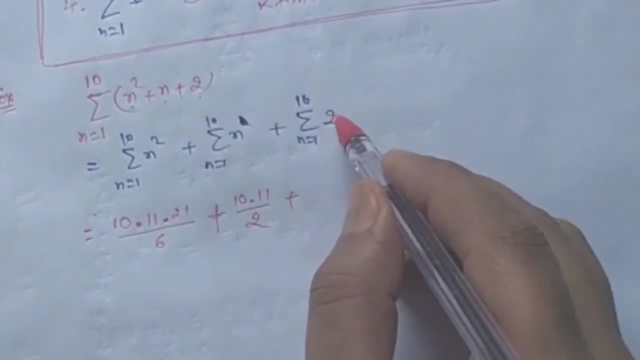 and what will be the value of this expression? we know the value of sigma 1, but we don't know the value of sigma 2. so now see in this, 2 is not dependent on n, so we can take out 2 just now. we have seen the third property. 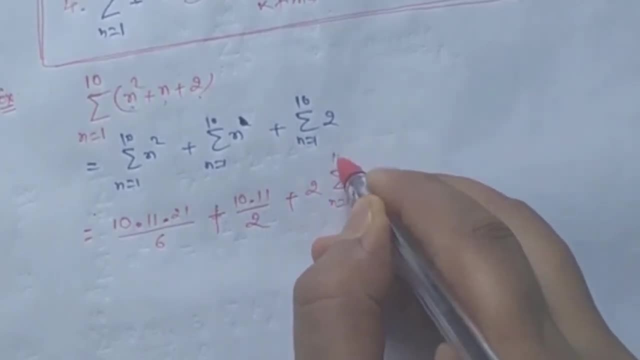 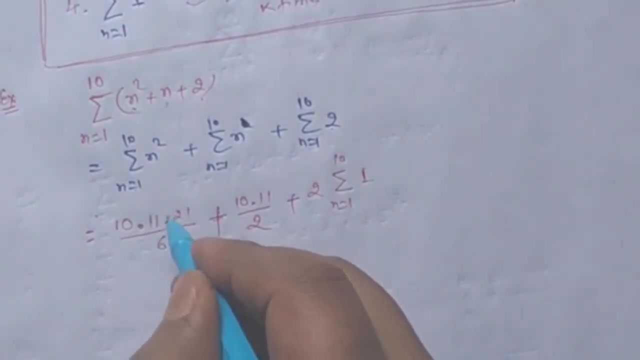 so we can write this expression: n equal to 1 to 10, and if we take out 2, then what is left, 1 from here terms will be cancelled. so we will cancel it and you will be able to solve. so how much is this? 55 into 7. 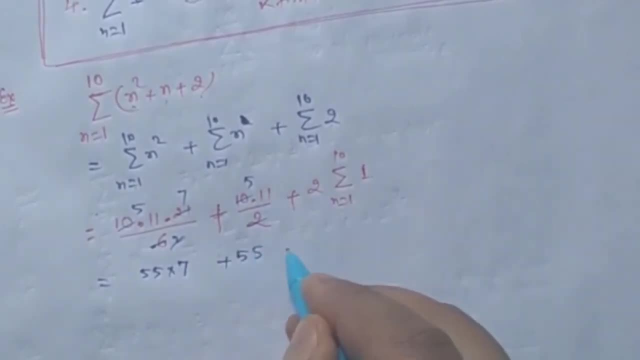 plus 55 plus 2 into sigma 1's value from 1 to 10. how much will it be? so see in the formula how many times 1 will be repeated: 10 times, and this expression came. now the simple addition of numbers, we can complete it. 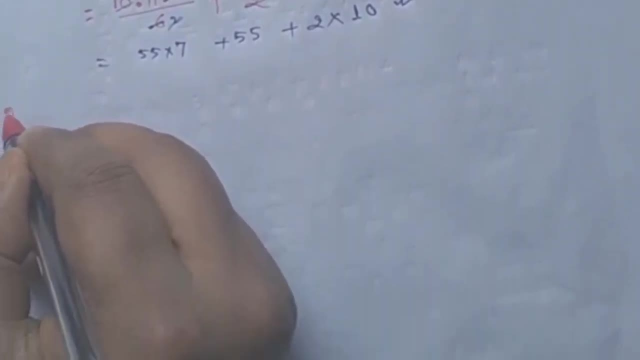 so some examples, some questions I am giving you. try it. how to calculate its value? ok, if this question is not there, then in the next class we will solve it like: first sigma n, cube, plus twice n, n, equal to 1 to 100. ok, question 2: 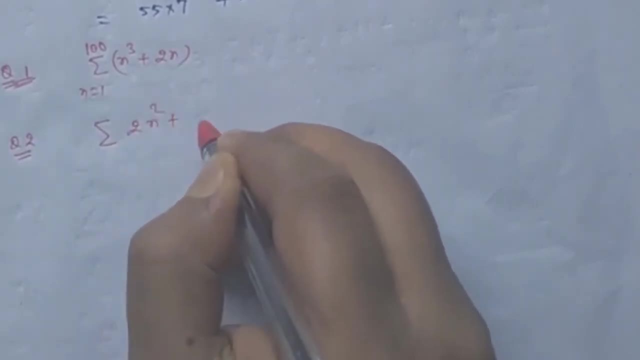 sigma twice n, square plus thrice n plus 5. so we are writing these 3-4 questions just for practice, so that you can solve the formula in a good way. ok, you have to try all these questions once and simple the property we have read. 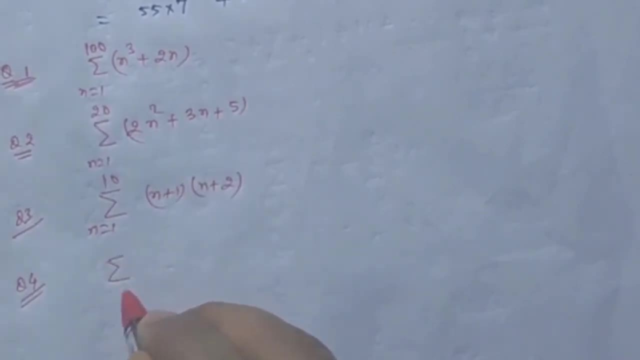 and the table we have noted. just use that to solve this question. ok, so all these formulas will be revised along with you and method. you will also understand how we are applying it. ok, just a little calculation will be more, so you have to keep that in mind. 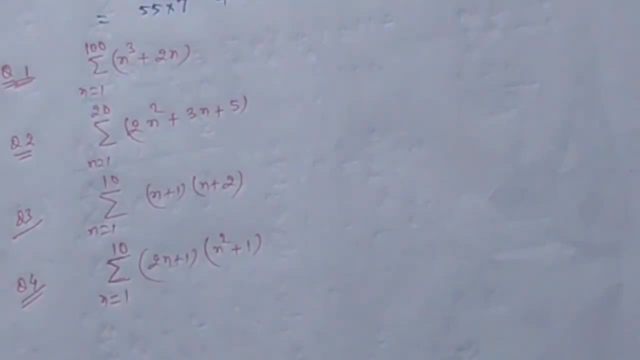 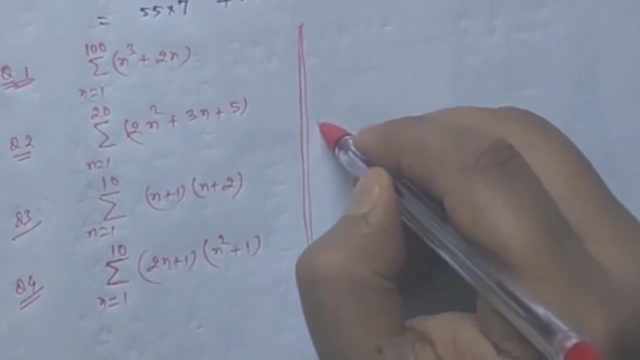 there will be no other problem. so these are 4 questions. you have to try these 4 questions. how to solve these 4 questions? ok, after this, in the next class, we will discuss this. if there is any doubt, then you raise the doubt. after that, we will discuss all these questions. 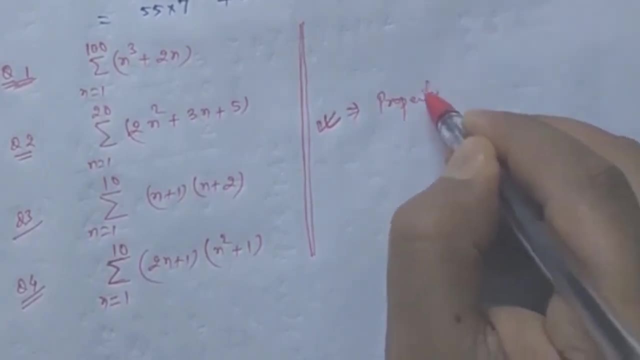 how to use the formula. so in all these questions we have written and the table we have noted. so we have to use that table in this. so this is on the basis of two tables. ok, so till here the notation part and in notation, basically the sigma part.